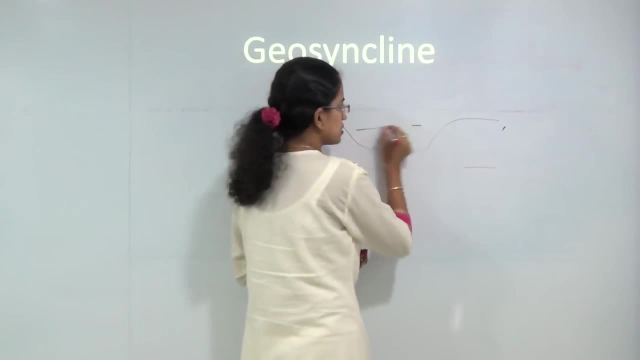 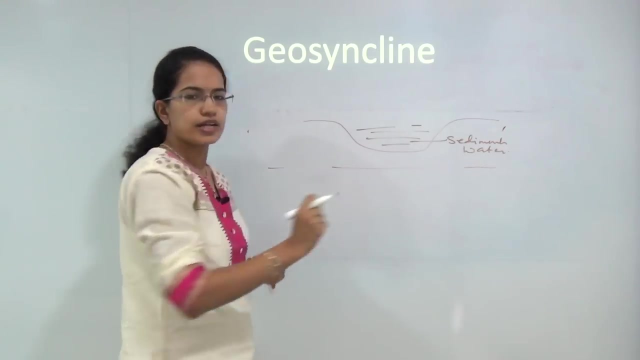 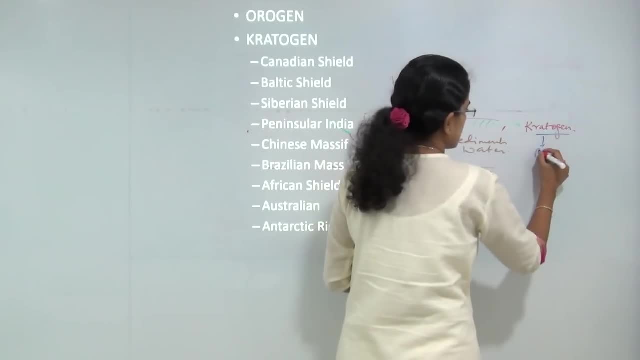 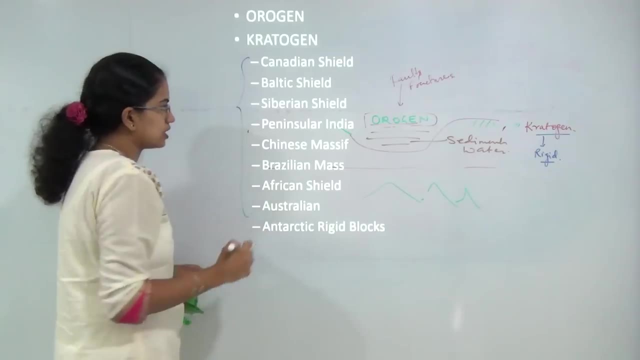 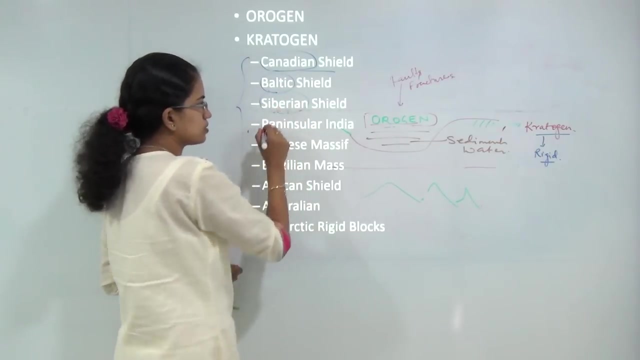 The sixth component is the geosynthetic material. The sixth component is the geosynthetic material, Cartogen, which is considered as a rigid mass Now across the globe. he mentioned few primary Cartogen areas. these were the Canadian shield, the region of Canada, the Baltic region. in Europe you have the Siberian region towards. 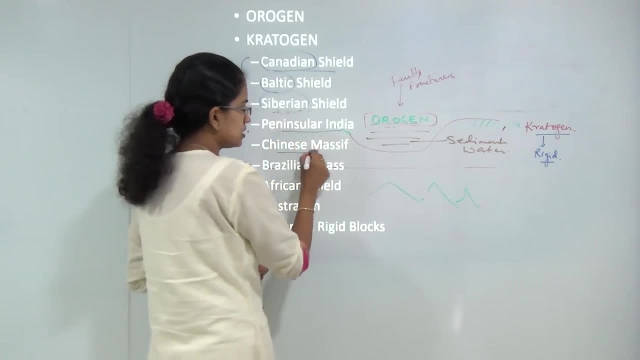 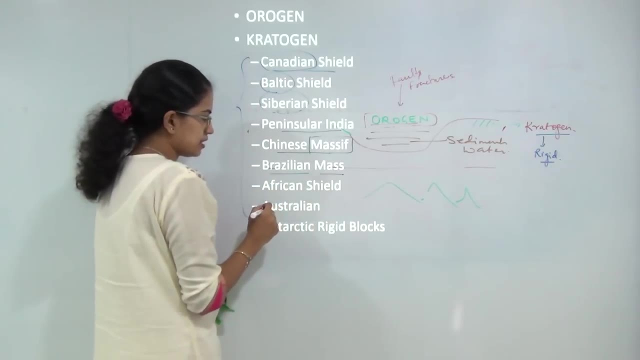 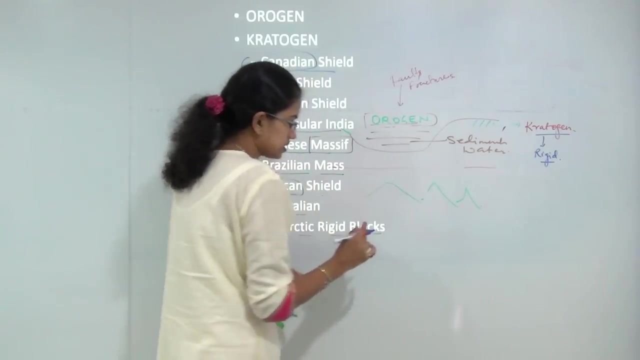 north, the peninsular region of India, the Chinese massive or the central plateau region of China, the region of Brazil known as Brazilian mass, the major central part of Africa known as the African shield. the Australian and the Antarctic rigid blocks were the regions 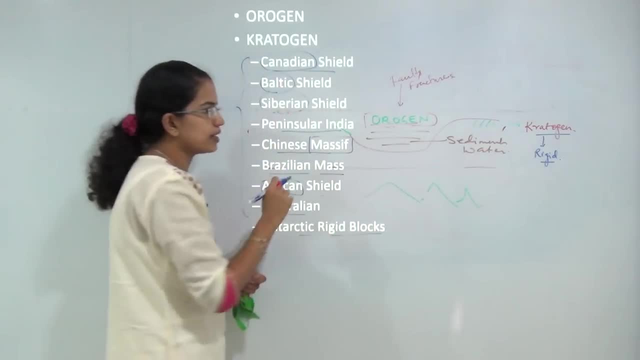 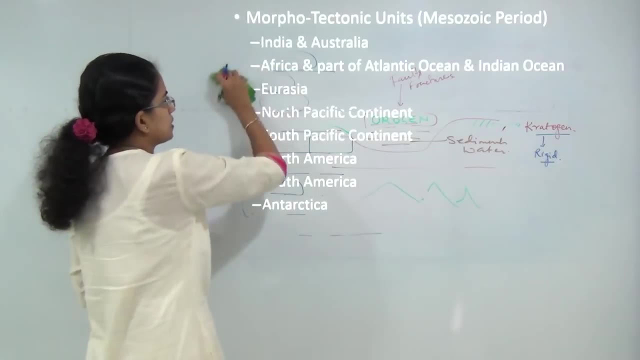 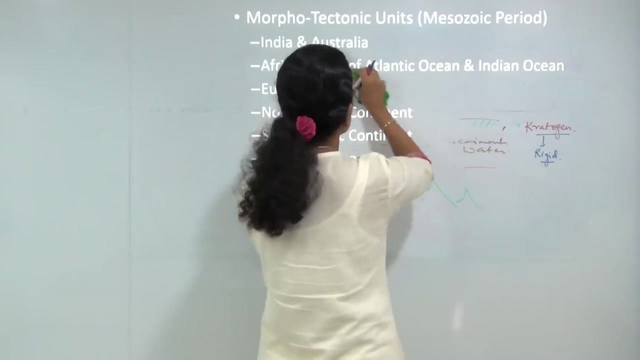 which were considered as Cartogen by Kober. So he talked about Orogen, he talked about Cartogen. The next thing he mentioned was the Morphotectonic units. Now, these were the units that are prone to tectonic movements, and along these units were 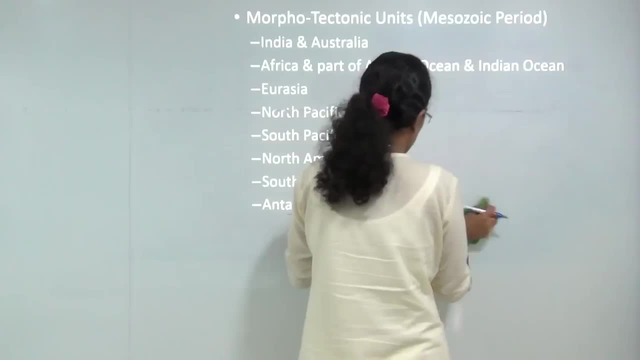 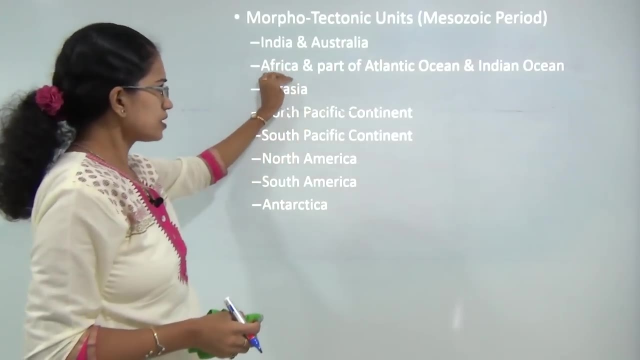 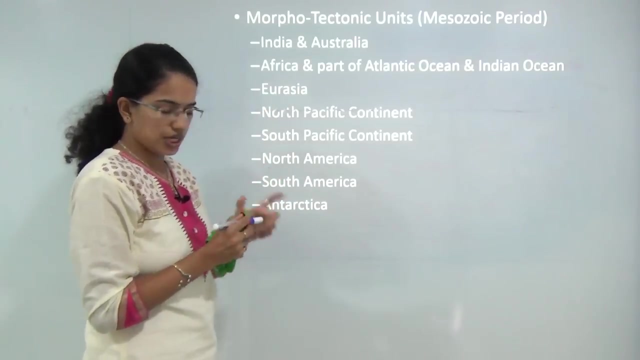 the region of China, The region of mountain building or the region where mountain building really occurred. So he mentioned the areas as the area of India and Australia, Africa, along with parts of Atlantic ocean and Indian ocean. you have the area of Russia and Asia. sorry Europe. 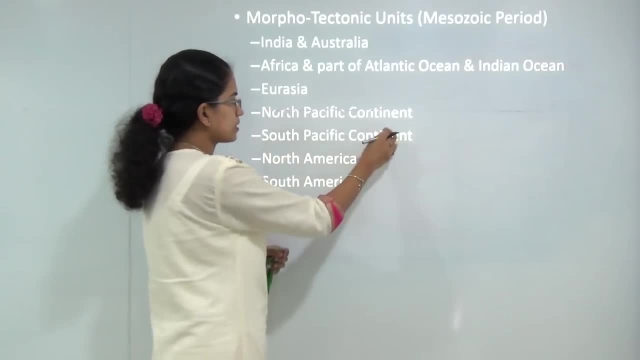 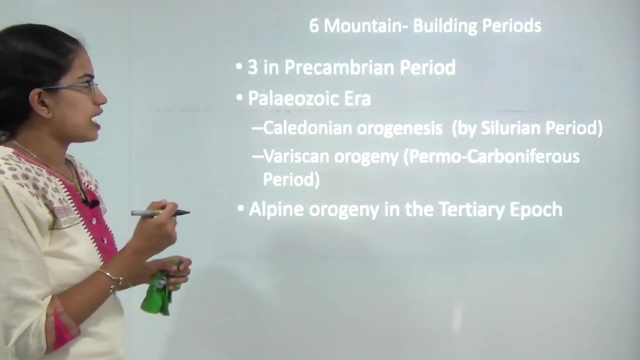 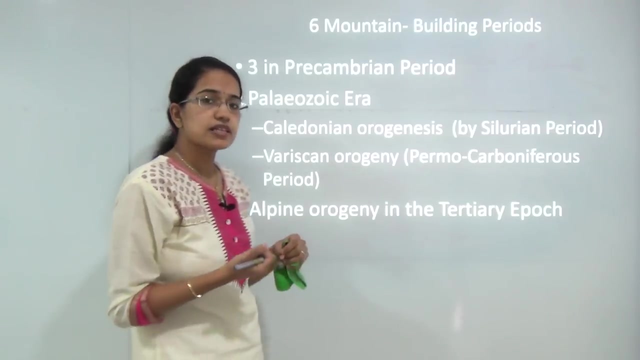 and Asia, known as Eurasia. Then you have the North Pacific continent, South Pacific, Northern America, Southern America and Antarctic area. Now let's understand how he tried to explain the concept of mountain building. So when he tried to explain the concept of mountain building, he talked about that mountain. 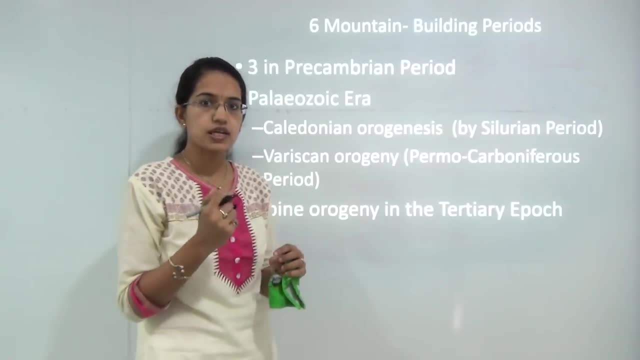 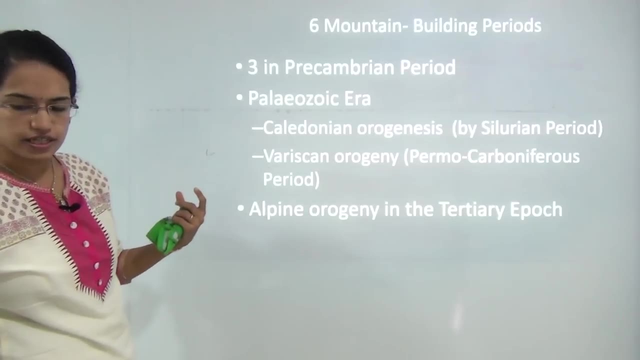 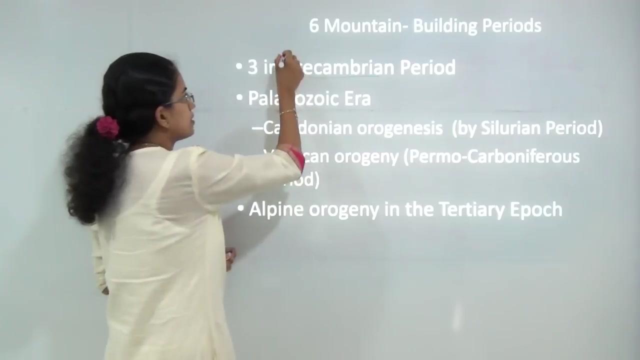 building was not an instant process. It was a gradual process and it occurred around series of periods that I should say. So he said that mountain building started during the Pre-Cambrian period and there were there were three mountain building periods that occurred during the pre-cambrian period. in all he focused. there were six mountain building periods, three of those light in the pre-cambrian period. the next was Paleozoic era, in which you had two major orogenesis cycle: one was known as the Varsikon cycle and the Caledonian cycle. this occurred during Silurian period, and this during the Permo-Carboniferous period. and finally, you have the most recent of the Alpine Orogeny, which resulted in formation of Himalayas and Rockies, and this was during the Tertiary epoch. so these were the basic mountain building periods that were highlighted. 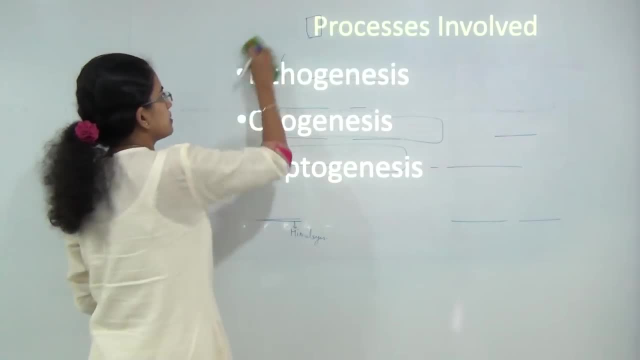 by Kober. now let's start with understanding the processes that were given by Kober. to begin with, what Kober said: Kober prepared the mountain building period for the pre-cambrian period in the pre-cambrian period. Kober prepared the mountain building period for the pre-cambrian period in the pre-cambrian. period, in the pre-cambrian period. in the pre-cambrian period, So Kober founded that there are forces of contraction which occurred due to cooling of earth and this lead to horizontal compression movements and this horizontal compression movements cause squeezing and that squeezing results in formation of mountain. that was 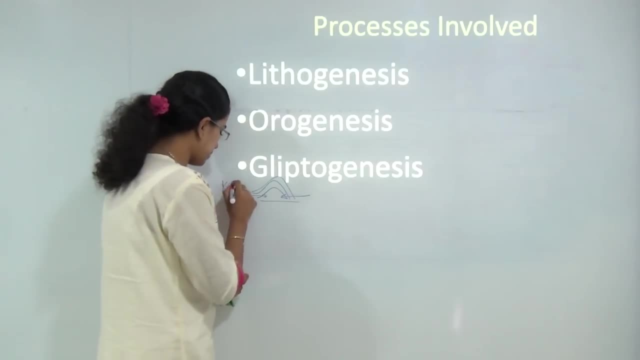 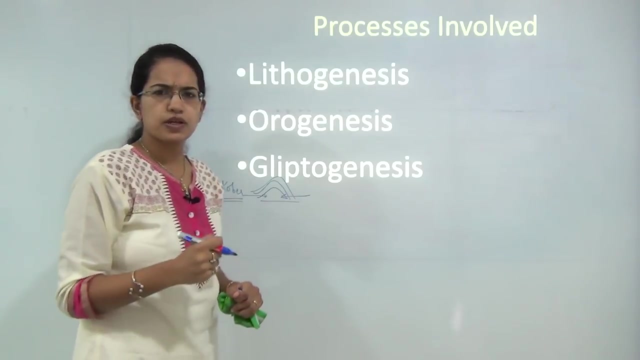 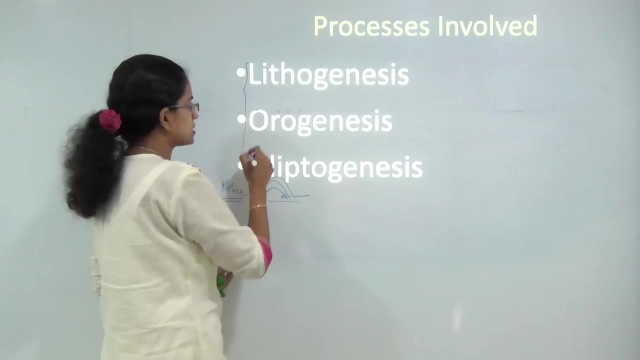 the basic thing that Kober try to explain Now. Kober, when he was explaining this concept, he brought about three terms when he was explaining which were most popularly used in and across all theories of mountain building. So he termed the three phases as Lithogenesis, Orogenesis and Glyptogenesis. 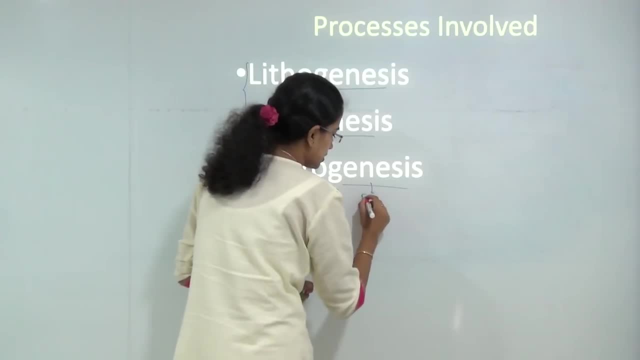 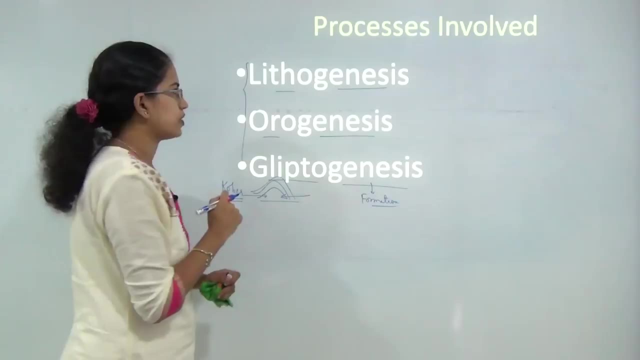 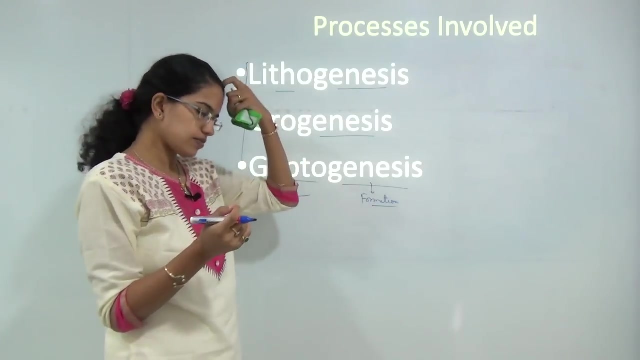 Now, the word genesis itself means formation. So in all the three stages we are talking about formation. Let's move on to each stage one by one. So under the first stage- that was Lithogenesis- he talked about that- there is contraction of the surface of the earth which is resulting from the cooling of the interior of earth. So, due to cooling of earth, what is happening is there is contraction and this contraction is causing the changes on the surface of the earth. So what is happening is towards the sides, where you have the folds or the crevices, the mountains, those try to scramble down and fall into the geosynthaline region and 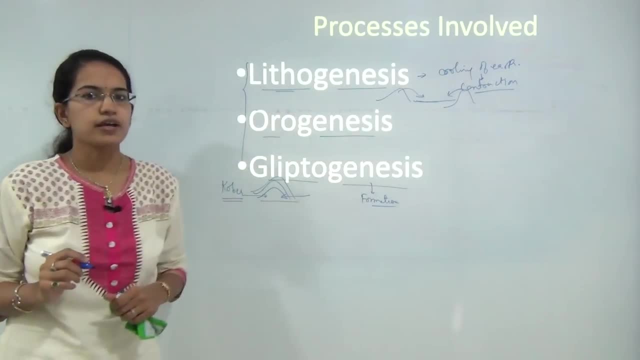 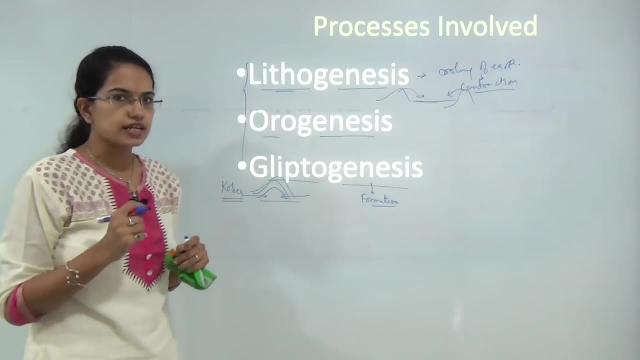 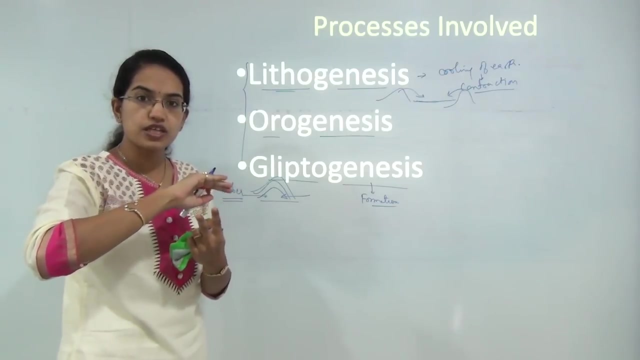 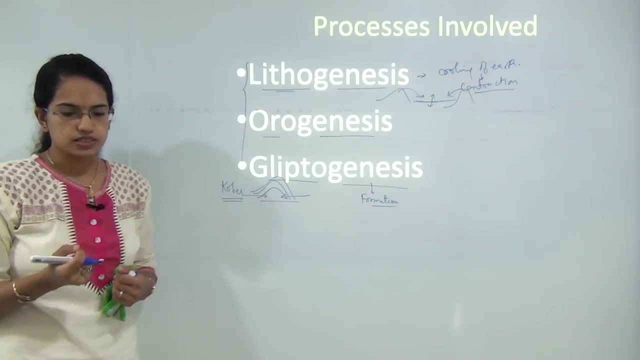 this is what was termed as Lithogenesis by Kober. Now, when Kober was explaining the concept of Lithogenesis, he explained a very interesting phenomena. He gave two things and he said: due to the result of these two things, there is increase in the thickness of this mass. and what were those two things? 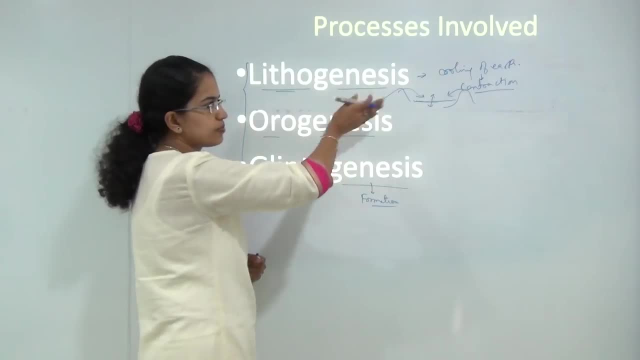 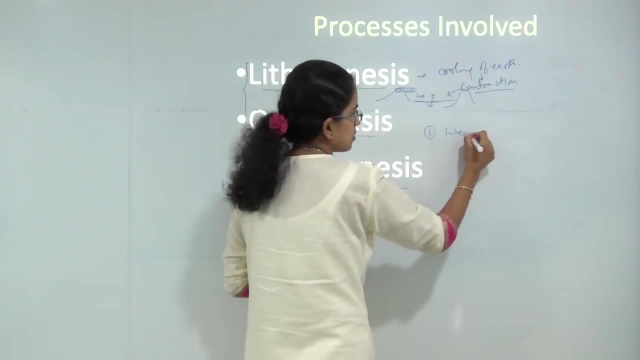 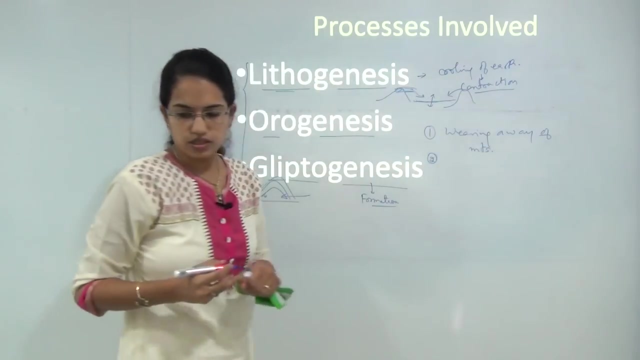 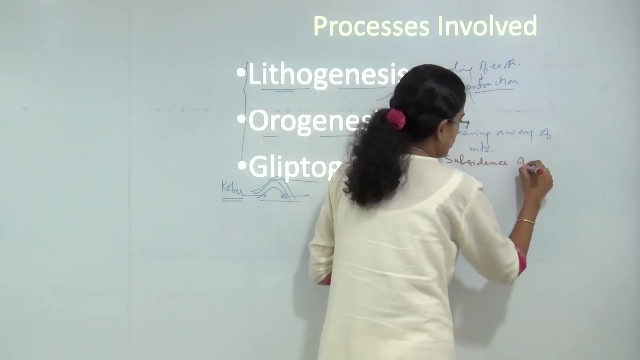 The first was wearing away of the fold and, as you can see, so the mountains are eroding and that is wearing away of the mountains. So one was wearing away of mountains, and the second was the subsidence of the geosynthaline, So you had subsidence of geosynthaline. 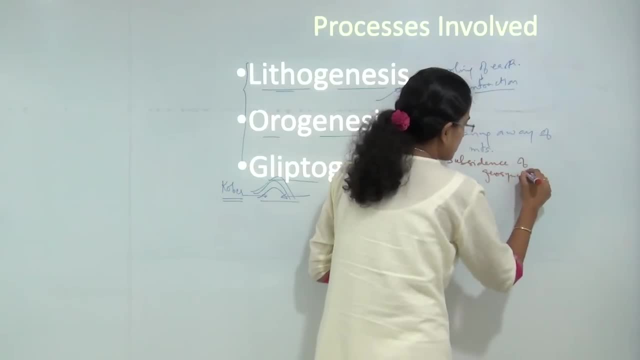 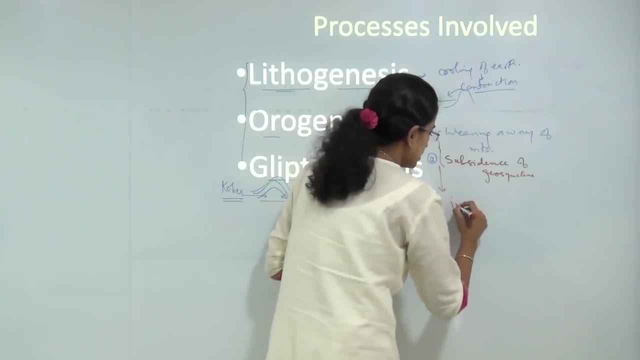 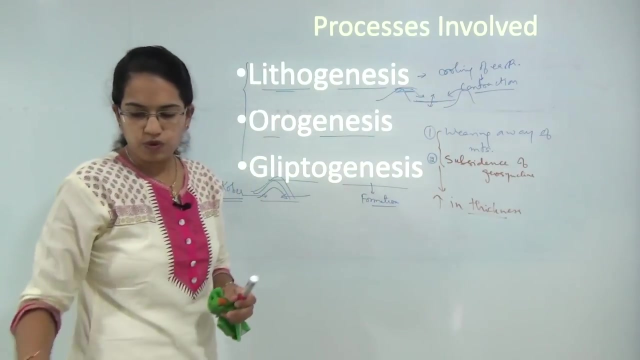 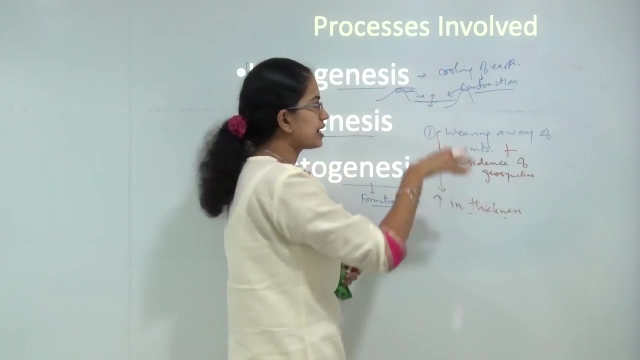 of geosinclined and because of these two, what happened was there was increase in the thickness of this geosinclined mass. so he said there are two forces which act together: one is wearing away of these mountains and the geosinclined going down and subsiding further because of 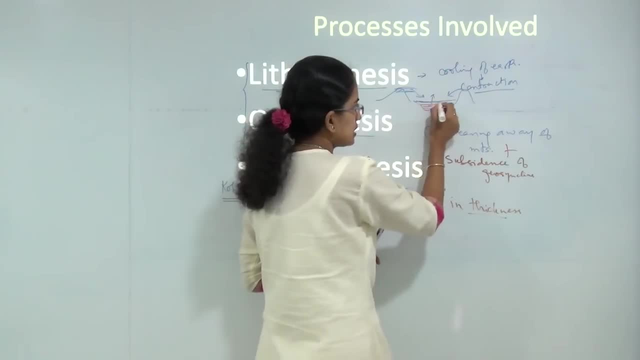 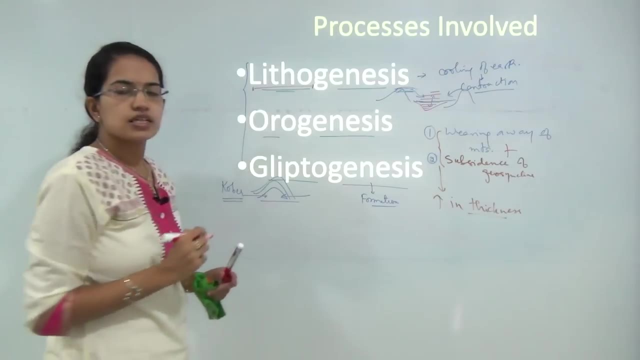 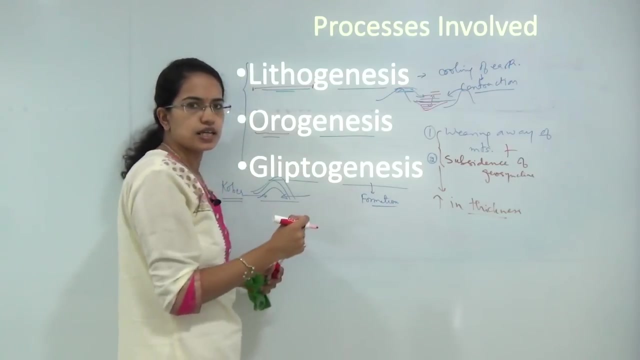 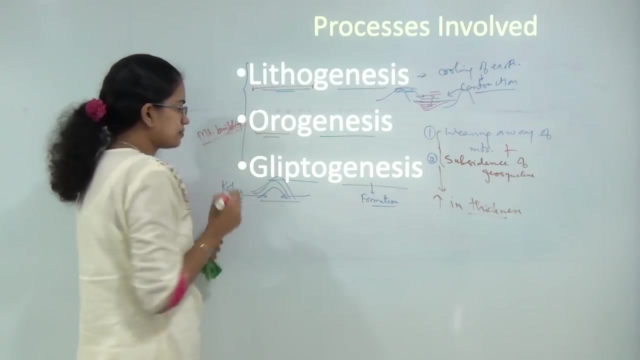 this. what happens was there is increase in the thickness of the deposits that occur here, and this was termed as lithogenesis. the next stage he tried to explain was orogenesis. orogenesis was the actual stage of mountain building, where mountain building actually took place. now to explain orogenesis, let's move on to a simple diagram. what gober tried to explain. 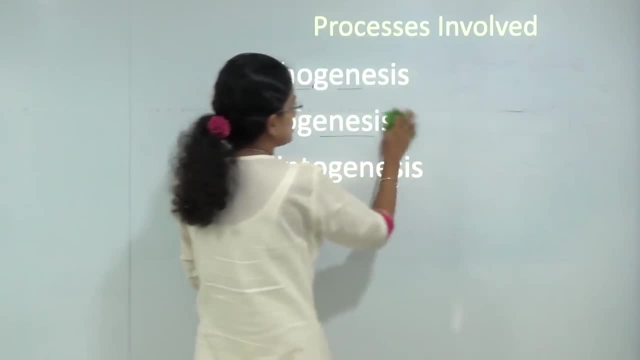 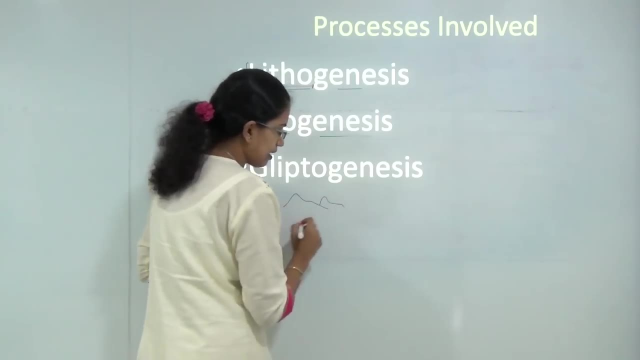 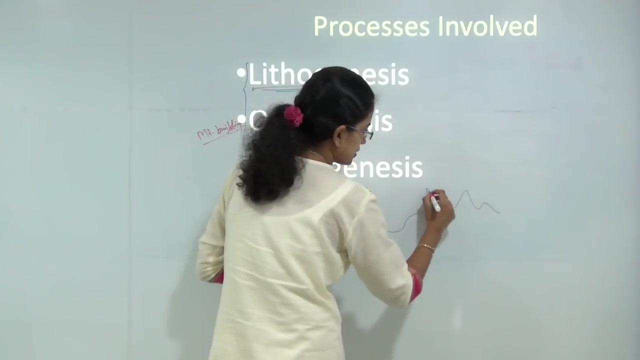 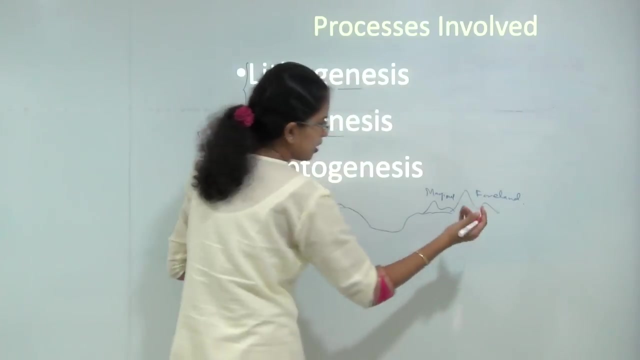 so, as we can see in all of his theories, you have the foreland, you have the marginal land, you have the geosinclined region, again the marginal land and the foreland. so this is, i could say, the marginal land and this is the foreland, or the stable block we also call 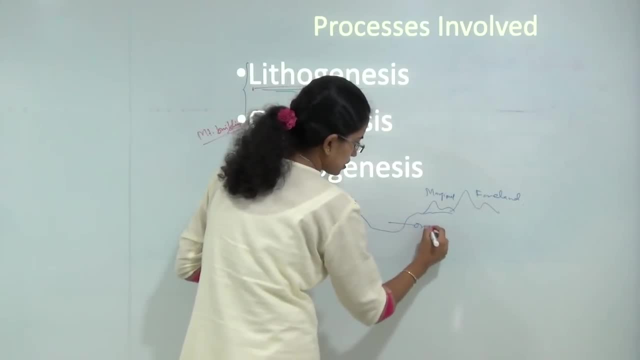 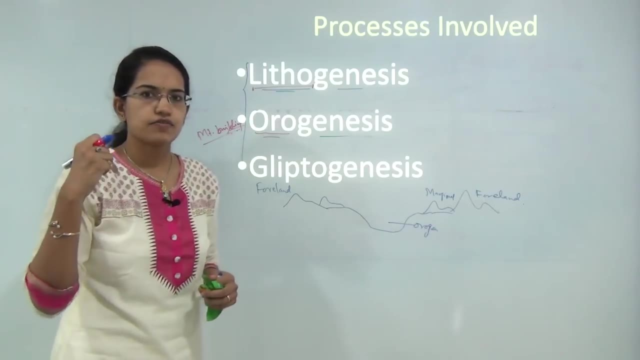 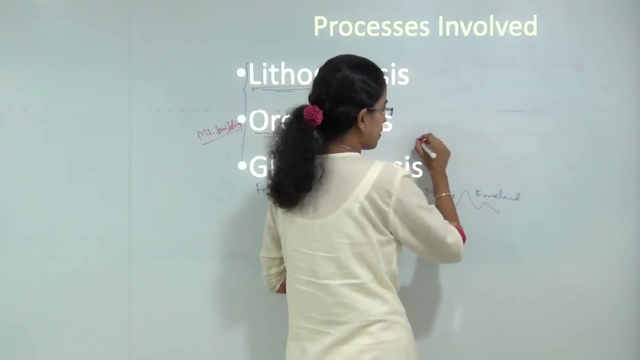 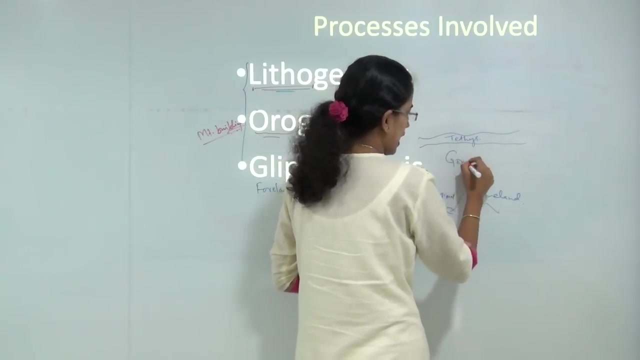 it cartogen, Now in the process of orogenesis. let's take a very simple example of the himalayan region. so i could say: you have the tethis river that was flowing. in the south the land was known as gondwana land and in the north it was known as angara land. 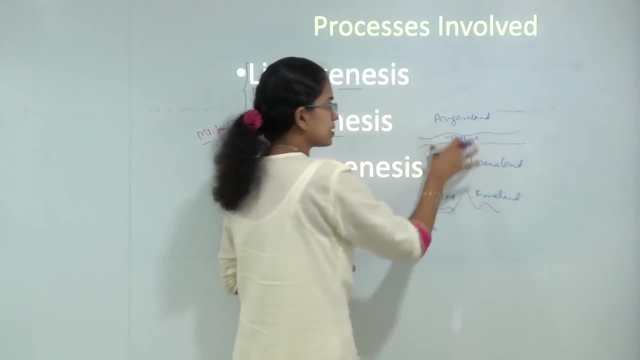 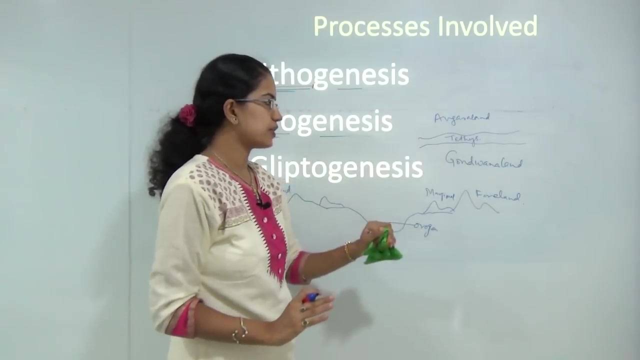 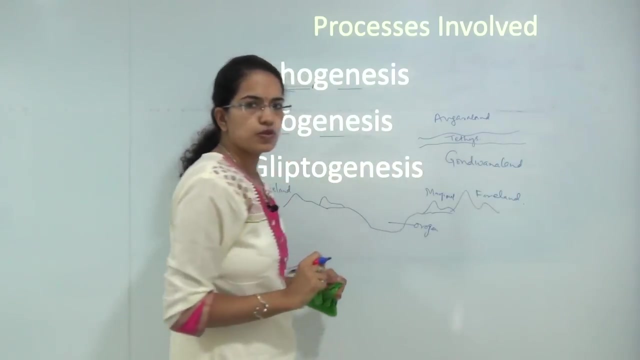 now this is something we would talk about in detail when we do the class on continental drift theory and plate tectonics. i am just giving you an introduction here. so you had the angara land in the north and gondwana land in the south. in the middle there was 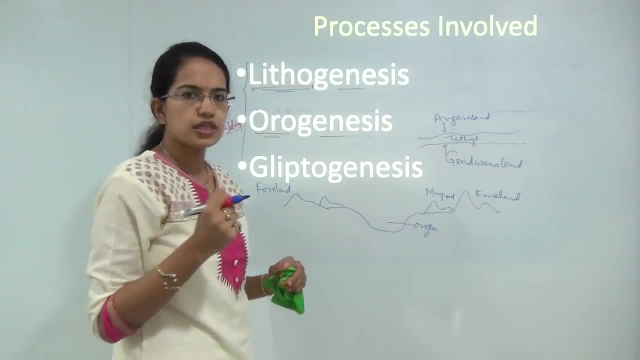 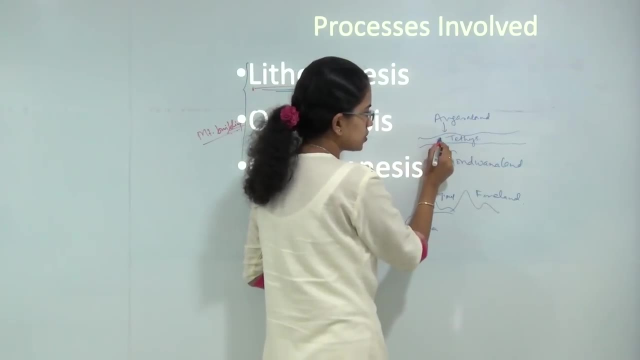 the river which was flowing, which was known as tethis. what he tried to explain was due to the compression forces from both the rigid land masses. here what happened was the development of Uhh, of the filling up of the geosyncline in this region. so this was considered as a geosyncline. 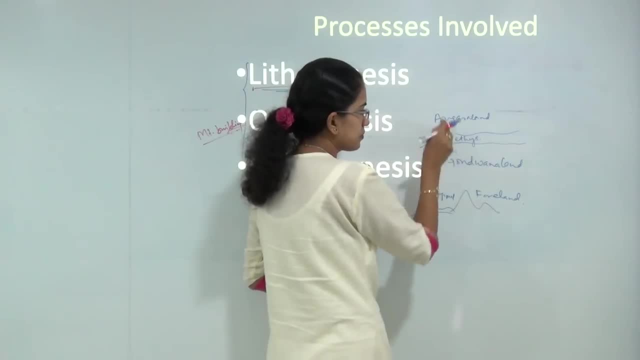 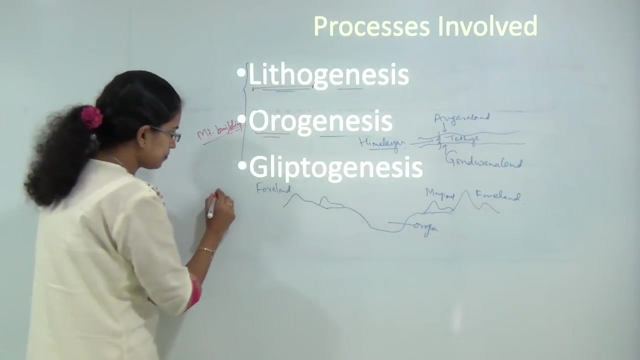 region and this region finally filled up with the subsidence and the wearing away of the solid, rigid blocks here that resulted in the formation of Himalayas. later on he tried to explain that you have the Himalayan mountain range and the Kunlun mountain range and in 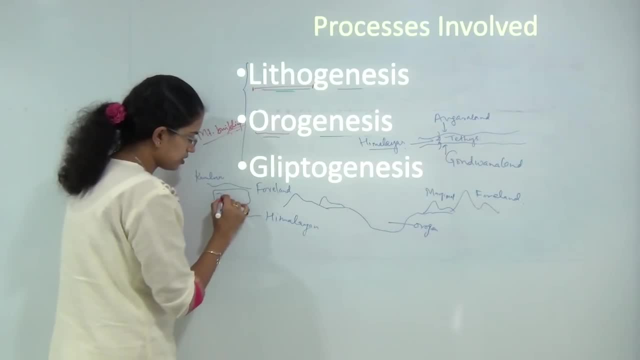 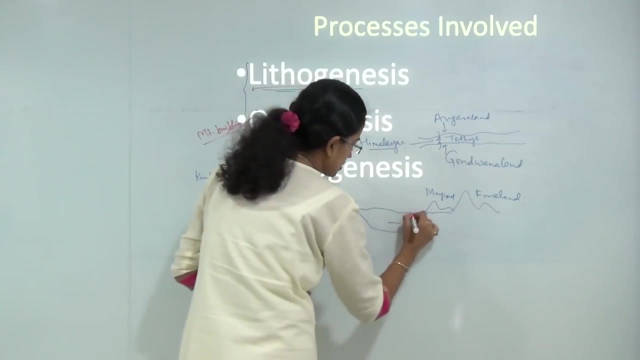 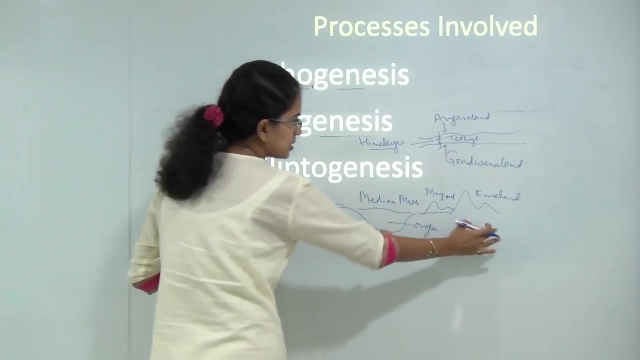 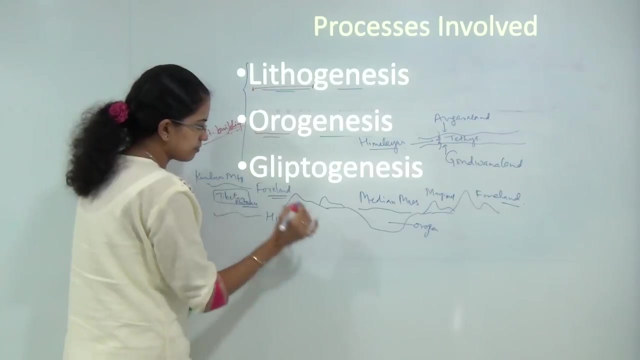 between the Himalaya and the Kunlun mountain range you have the Tibetan plateau, so he tried to explain this region as the medium mass, and across this medium mass you have the four lengths or the region of actual mountains. So you have Kunlun mountain range on one side, you have Himalayan mountain range on. 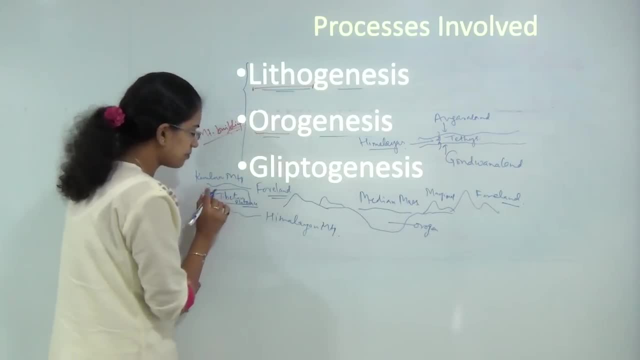 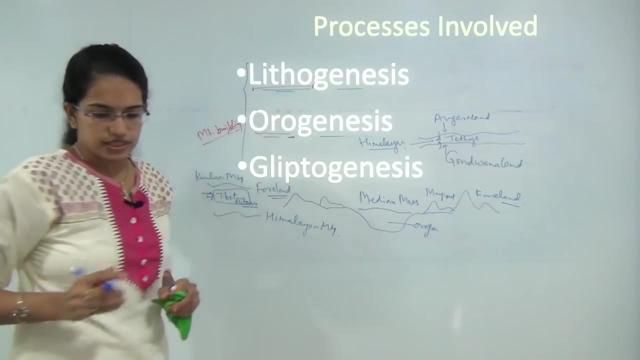 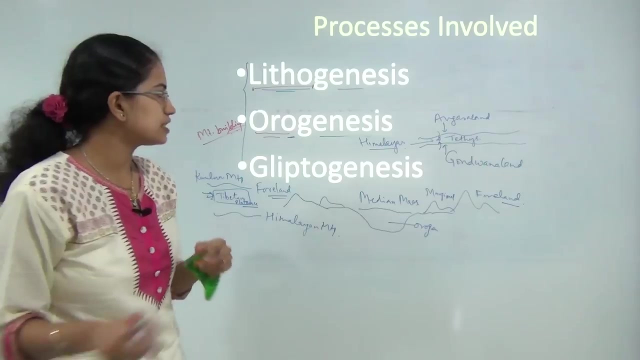 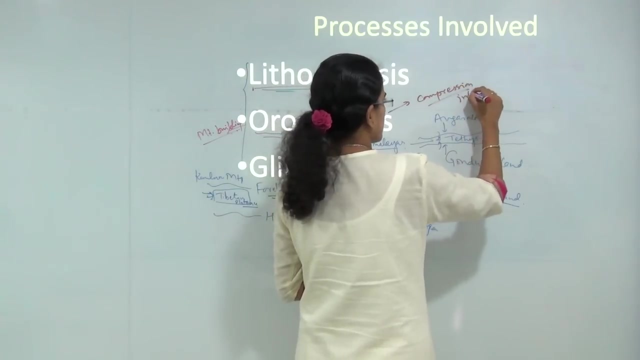 other side and the middle median mass was known as the Tibetan plateau. that is a classic example we can give to understand the cobers theory. So under the process of orogenesis, as I said, there was convergence of the intensity of compression, So the intensity of compression was very high. as a result, you had formation of huge 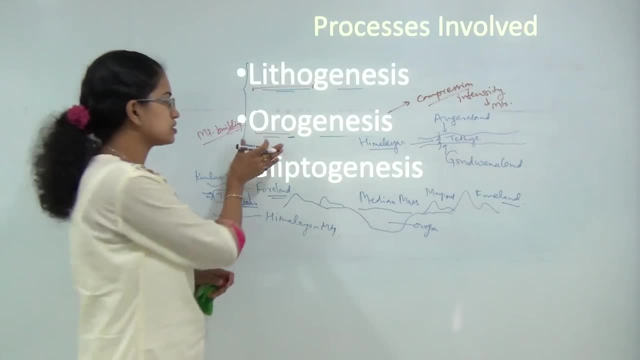 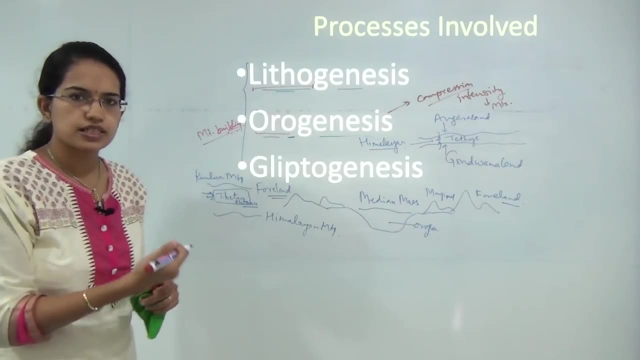 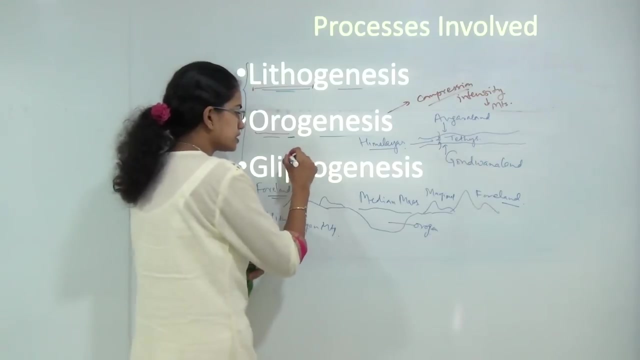 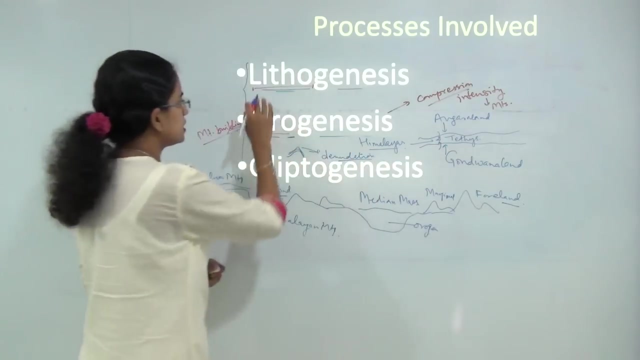 mountains. So that was what he propounded under orogenesis and finally, under glyptogenesis, he said: you have denudation that is acting and there is gradual decline or the gradual ascent of mountains that is taking place, which is very gradual, Along with the denudation processes that are acting up. so these were the three stages. 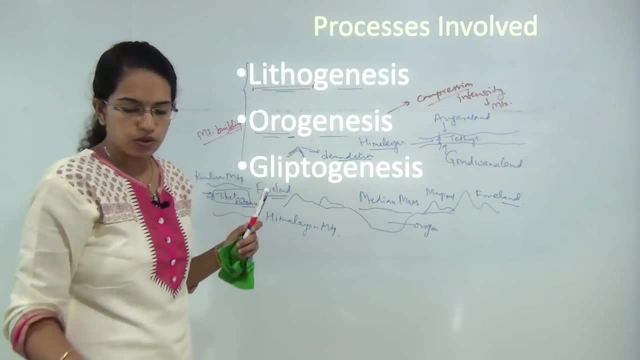 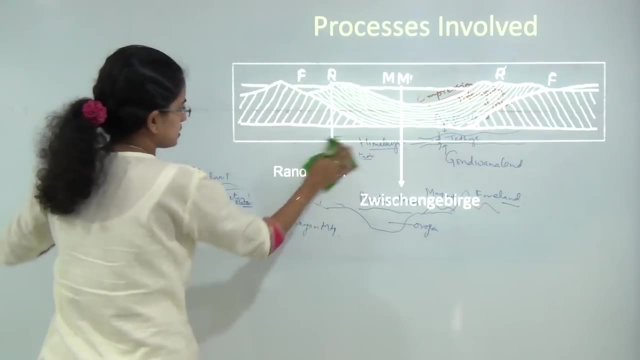 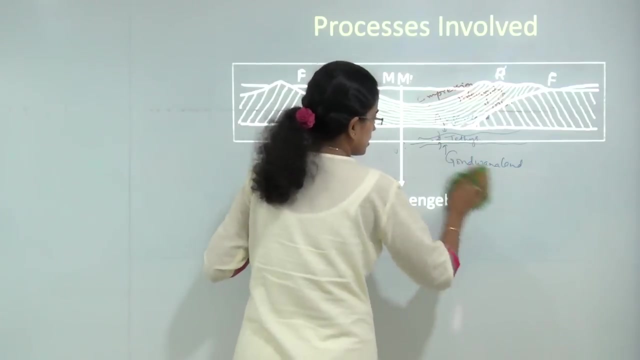 that he tried to explain to help understand the process for orogenesis. So here we can see: the region which is marked F is the fold end, as I explained here. then you have the marginal ranges, which are also known as Rankettin, and finally you have the 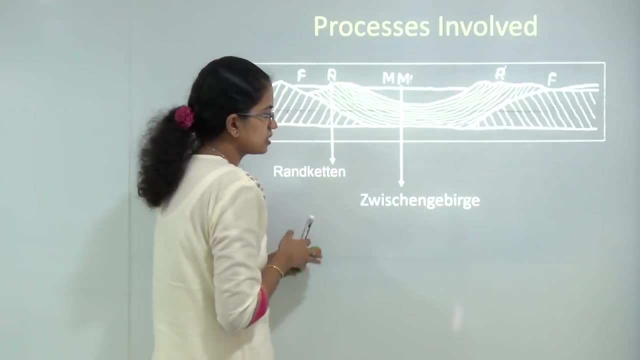 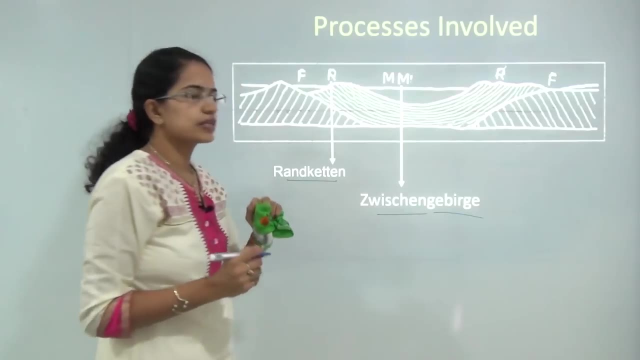 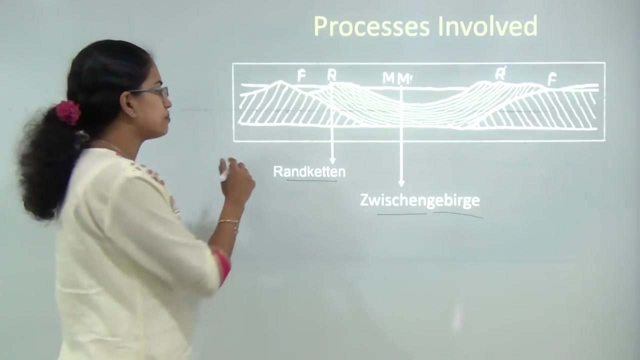 median mass, So between the two ranges, which was known as Jvissingibirt. so these were the terminologies that were used by Coburn to explain the concept and the process of origin of mountain building. Now, there were numerous examples that proved that this theory was valid. 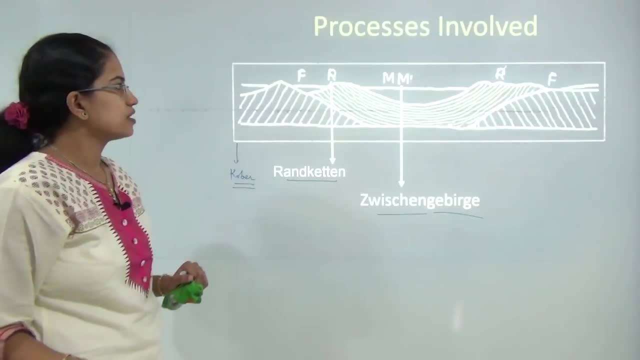 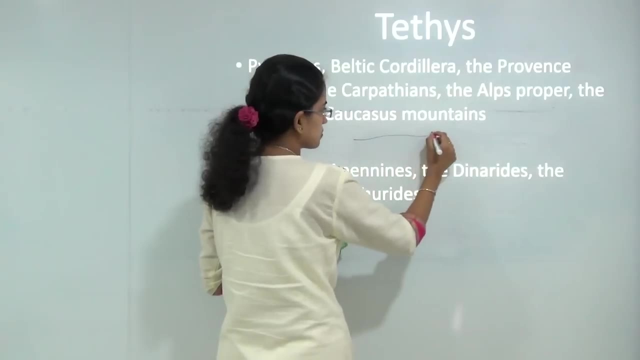 So if we move across the globe, we will find n number of examples. so let's first start with the tethys itself, which we were trying to explain. So let's start with the tethys itself. So you have the Tethys, you have the Angara land and the Gondwana land. 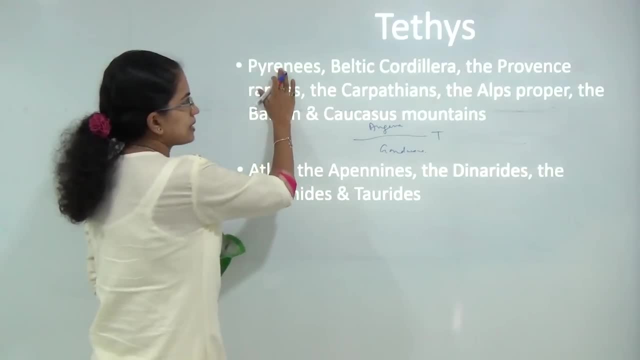 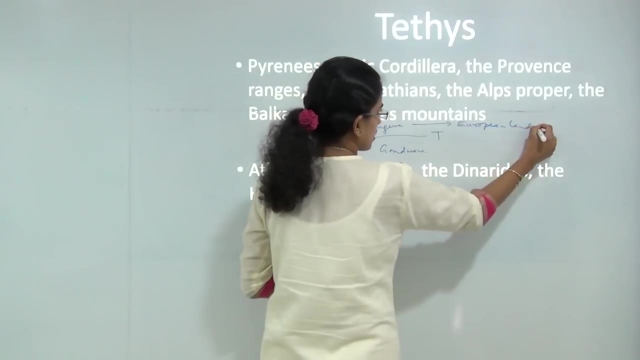 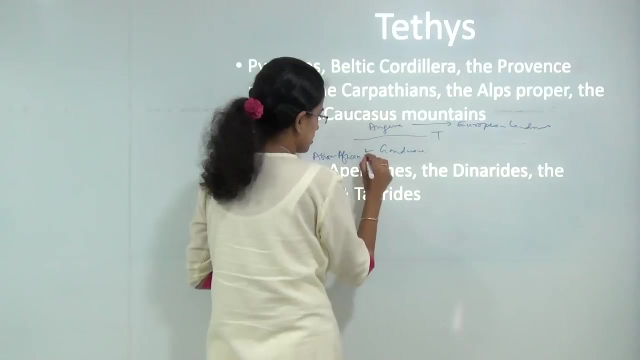 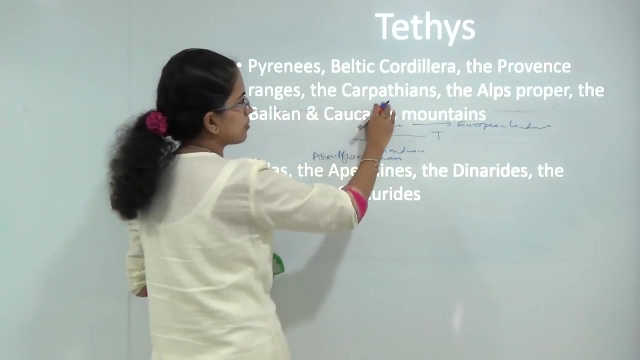 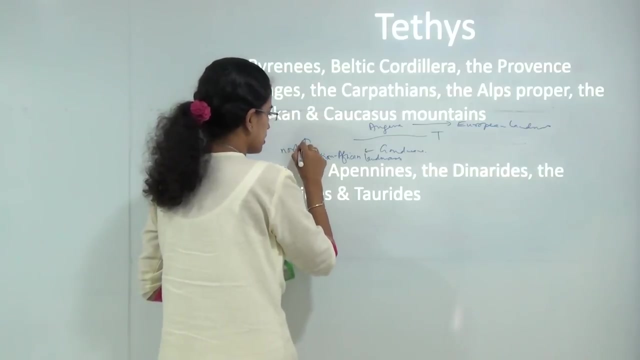 So what he said was Pyrenees, so Angara land- I could mark it as the European land mass and this would be the Asian African land mass. So what he explained here was range: Carpathians, Alps, Balkans and Caucasians were the result of northward movement of the 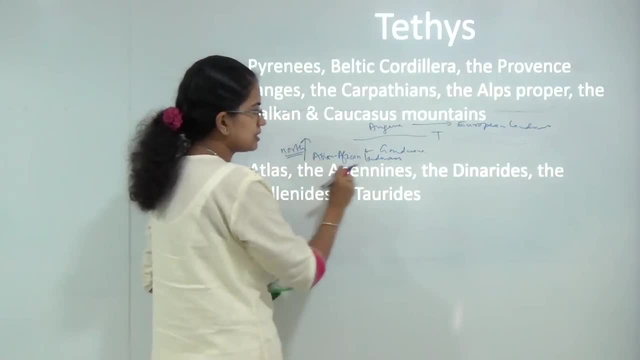 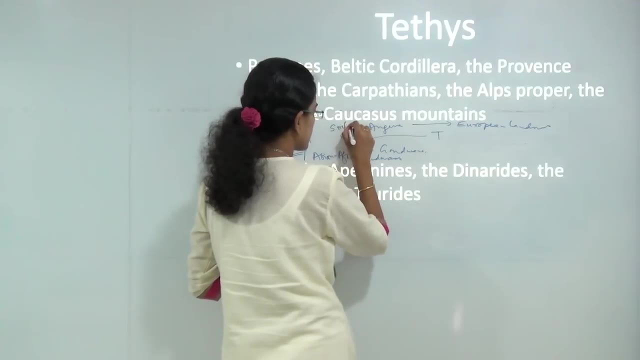 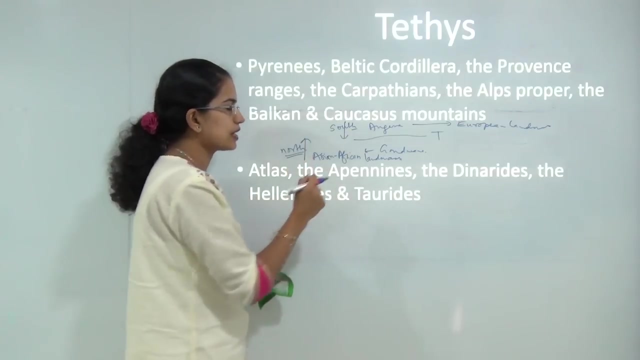 African landmass. In contrast to that, Atlas, Alpines, Dendrix, Hellenes and Tardis were the result of southward movement of the European landmass. So within a single process you had so many mountain ranges that originated. some of those 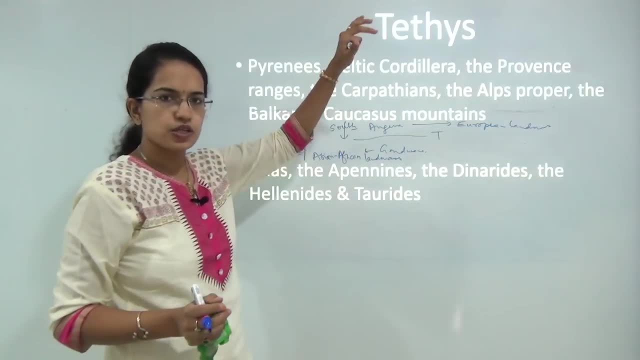 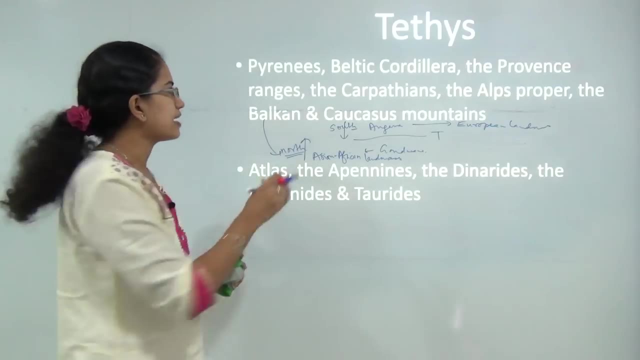 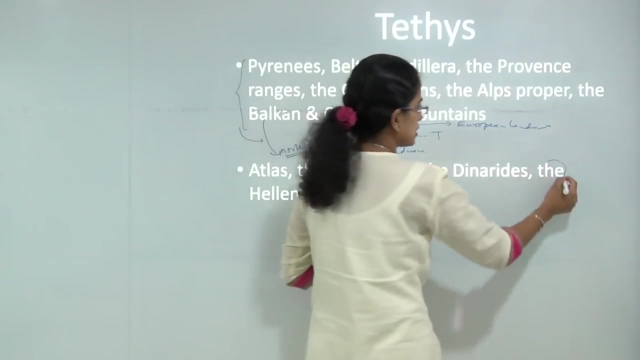 were the result of southward movement of the European landmass and some of those were the result of northward movement of the African landmass. So all these resulted due to northward movement of the Asian African landmass and all these resulted due to the southward movement of the European landmass. 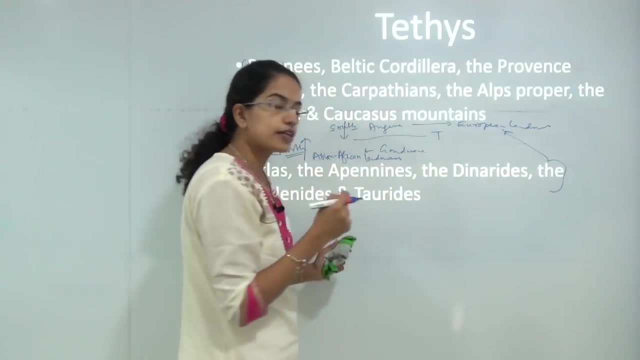 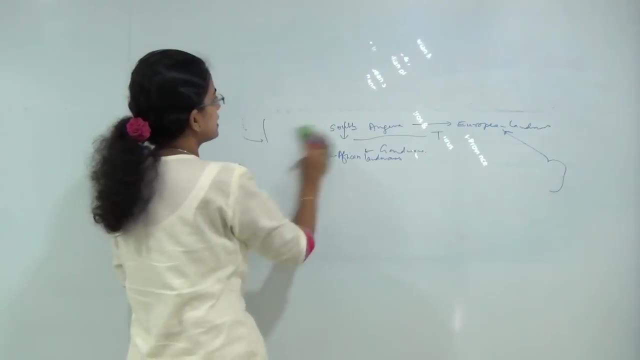 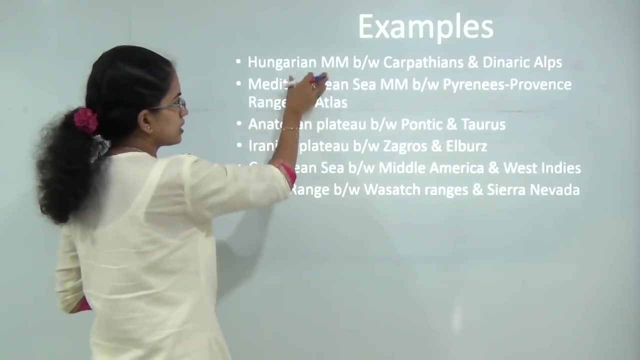 So that is one. when we talk about The Tethys Sea, we already talked about the Tipetan plateau lying between the Kunlun range and the Himalayan range. Some other examples which are most commonly proved by the Cobar's theory are Hungrian. 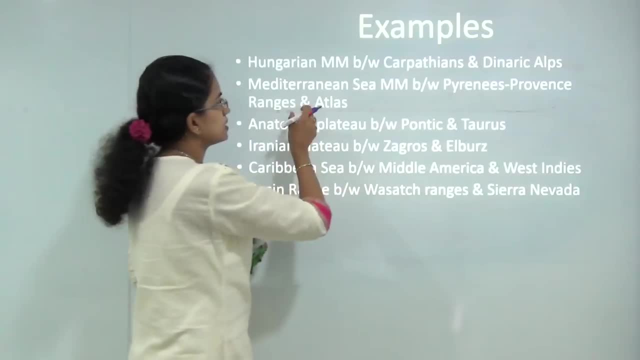 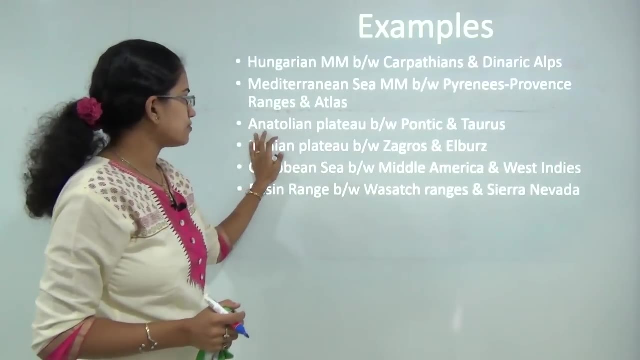 median mass, which lies between Carpathian and Dendrix. then you have the Mediterranean Sea that lies between Pyrenees in province in the north and Atlas in the south. Then you have the Anatolian plateau that lies between Carpathian and Dendrix. 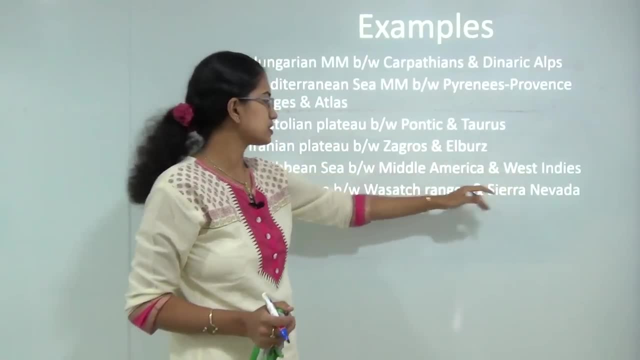 Then you have the Mediterranean Sea that lies between Pyrenees in province in the north and Atlas in the south. Then you have the Mediterranean Sea that lies between Pontic range and the Taurus range, Iranian plateau lying between Zergose and Elbrus range. 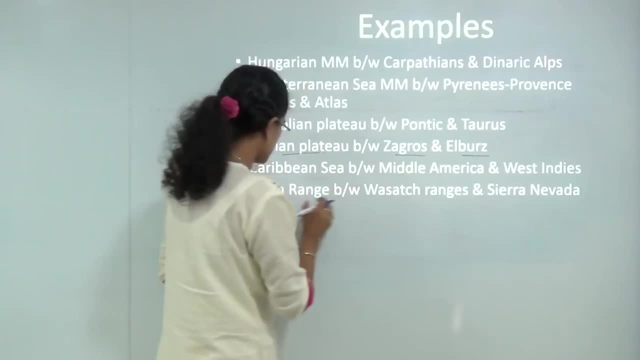 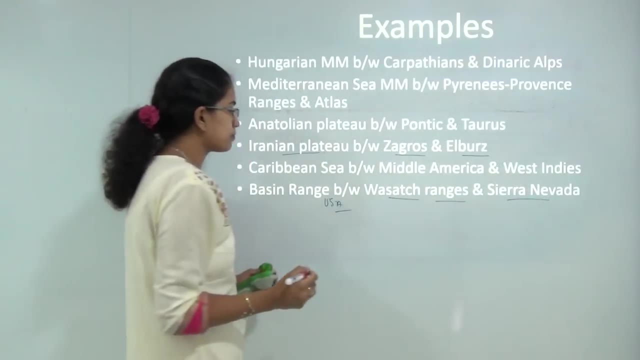 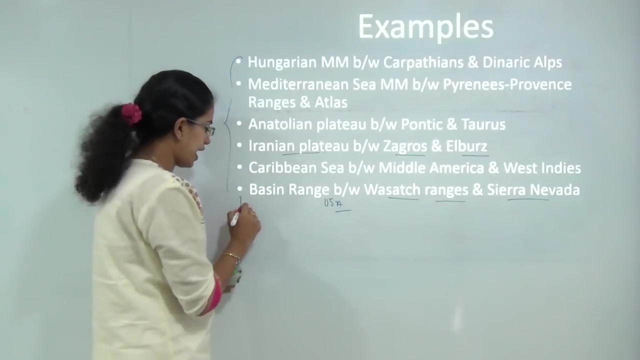 You have Caribbean Sea lying between Middle America and West Indies, and finally the Basin range in United States that lies between West Forge range and Syrian Aveda. So these are some of the common examples that we can lay down to prove that the Cobar's 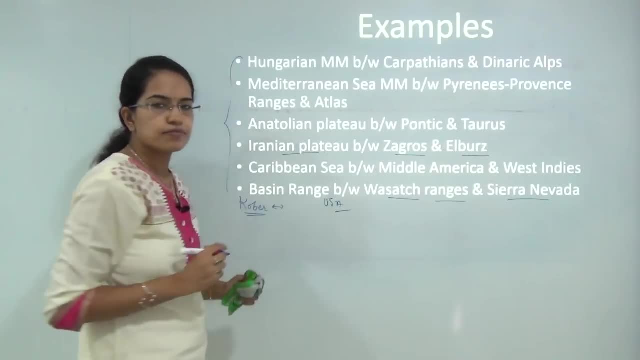 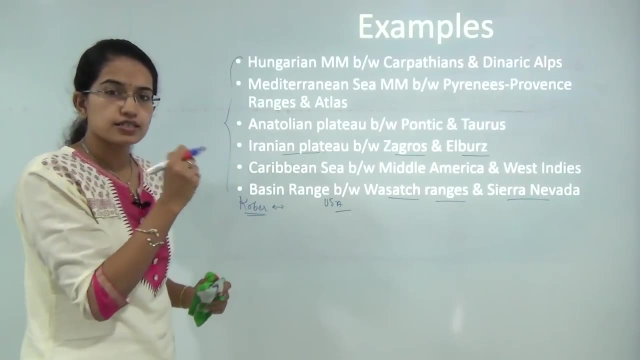 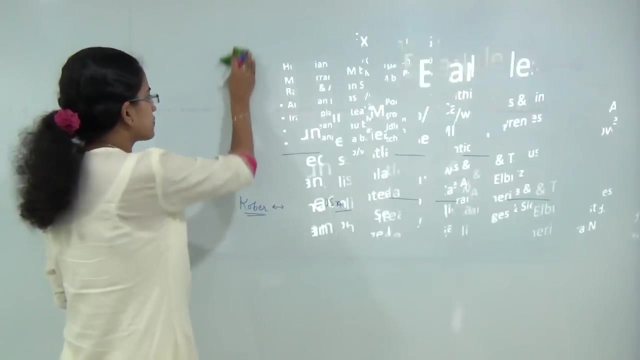 theory was a kind of valid theory in mountaineering. But despite of the facts that prove that this theory was considered as the most important and most popular theory among the mountain building theories, there were n number of critics that were raised to against this theory. So the first critic said that just the forces of contraction are not sufficient for formation of huge mountains like Himalayas or Alps. So that was the first part. Okay was the first controversy that it fell into. the next controversy was brought forward by Seuss. 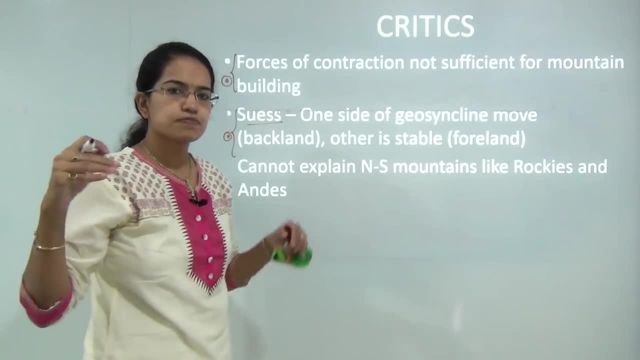 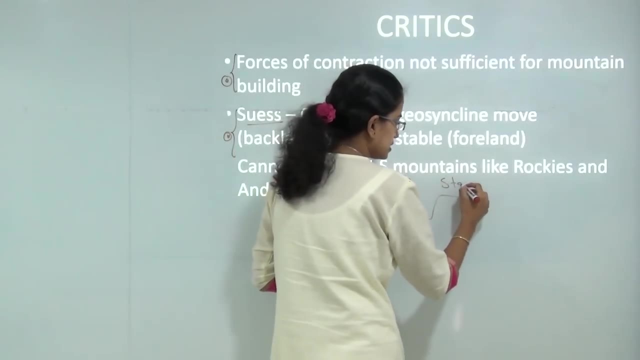 Seuss explained that whenever there is two land masses that exist, out of these two land masses one land mass remain stable, while only one land mass moves. So the land mass which is stable is known as fore land and the land mass that moves is known as back land. 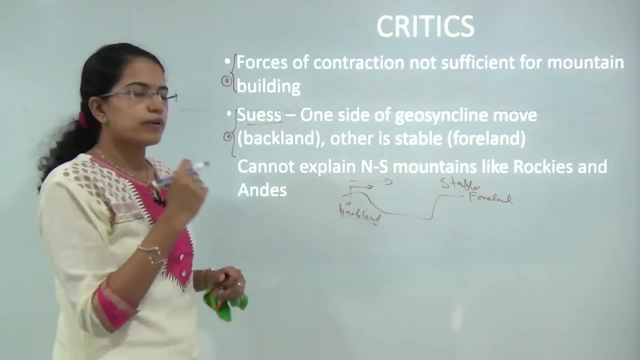 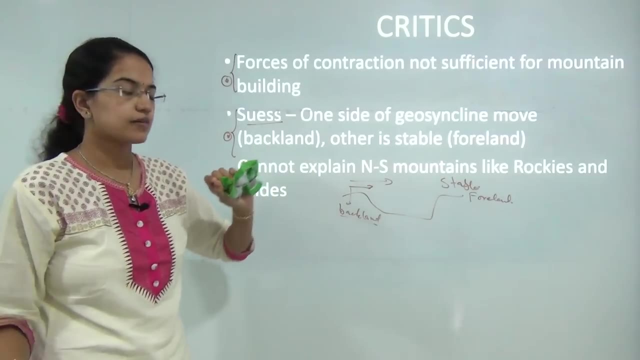 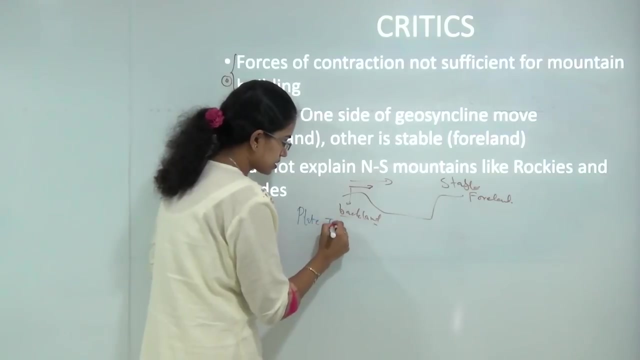 Seuss tried to explain that cobalt theory is not valid because it's only the angara land that is moving, while the gondwana land remains stable. but as and when plate tectonics theory came into discovery- and by the plate tectonics theory it was revealed that all 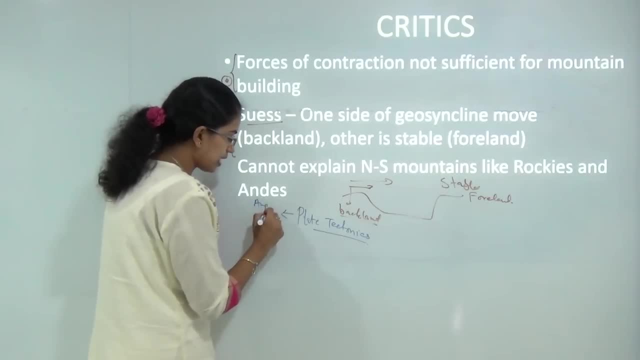 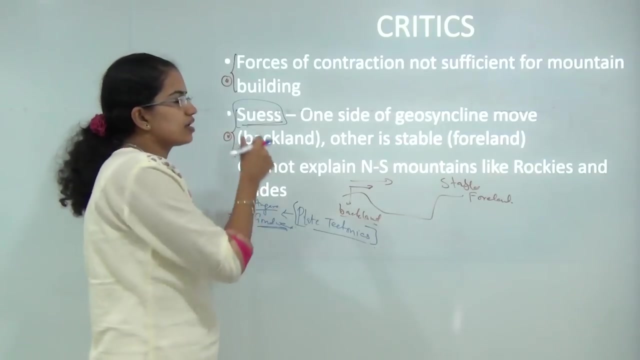 plates move, and it was not only the angara land that was moving, But gondwana land also started moving. So cobalt theory became valid again after the results that were driven from the plate tectonics theory Till then. Soess tried to provide a critic for this theory, and finally all the examples. 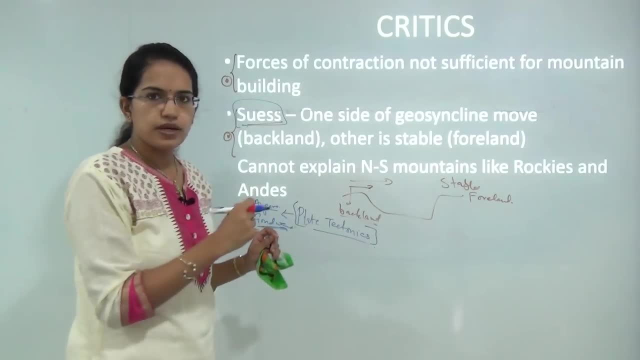 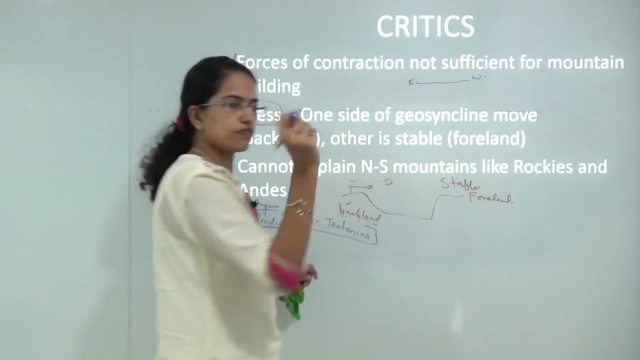 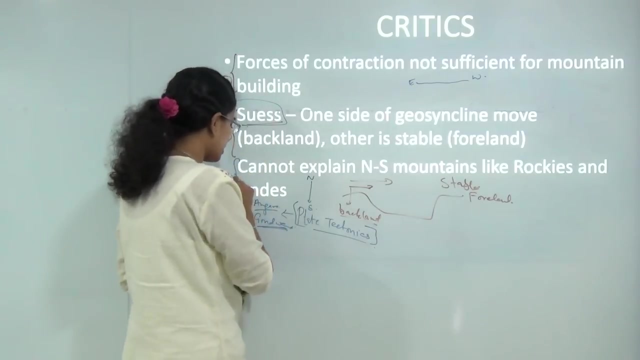 we have discussed so far, based on the cobalt theory, are all examples of the mountain ranges which run east and west. None of these examples could prove a mountain range that run from north to south. So this was again a major criticism that was driven for against the cobers mountain building. 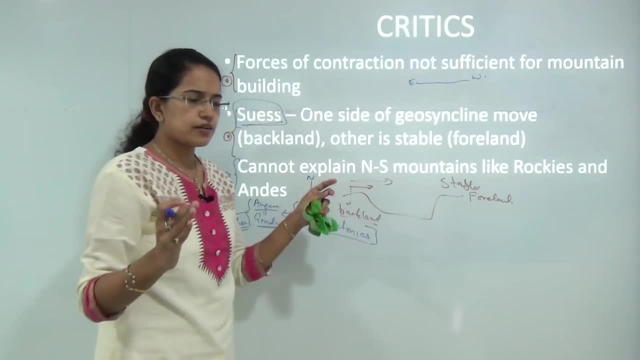 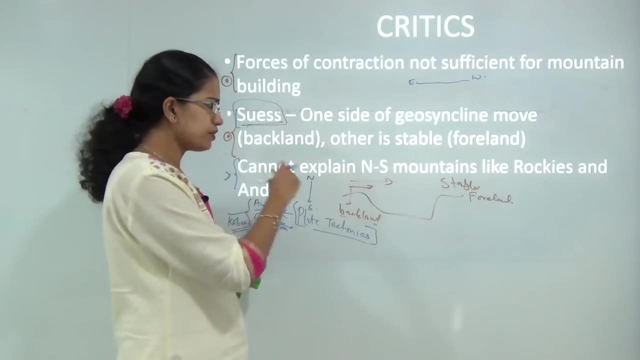 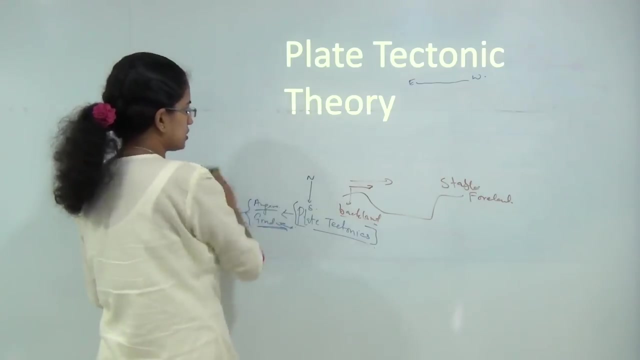 theory Now intermediate to cobers theory and plate tectonics theory. there were n number of theories. We would be discussing those theories in the further class. For now we would be straight forwardly moving to the plate tectonics theory for mountain. 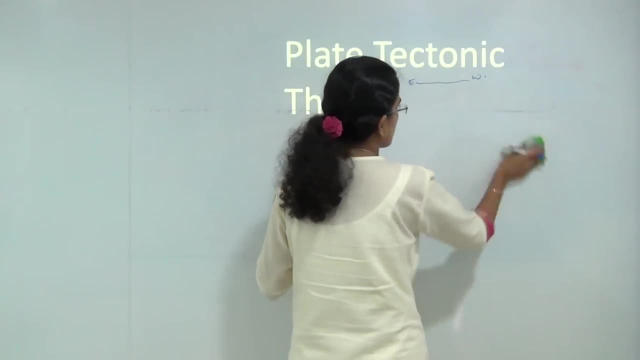 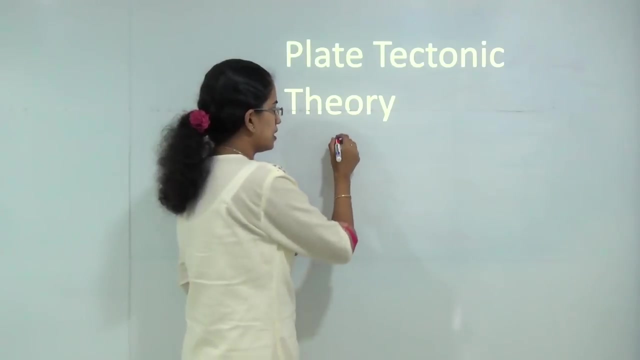 building, which is considered another major theory in terms of mountain building. Now, plate tectonics: the concept itself we would be discussing in a separate class. So for now I would be just introducing the three terms that we use under plate tectonics. 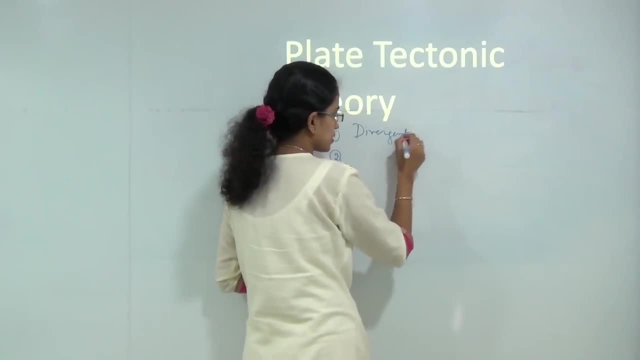 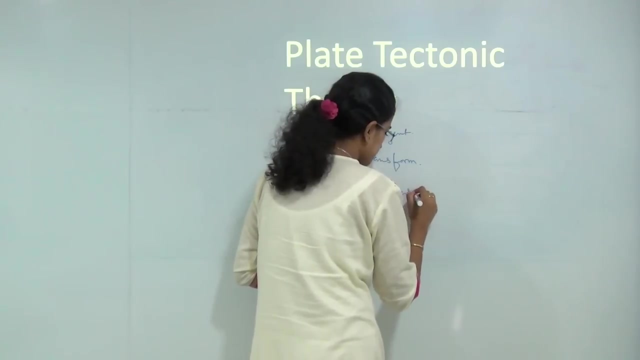 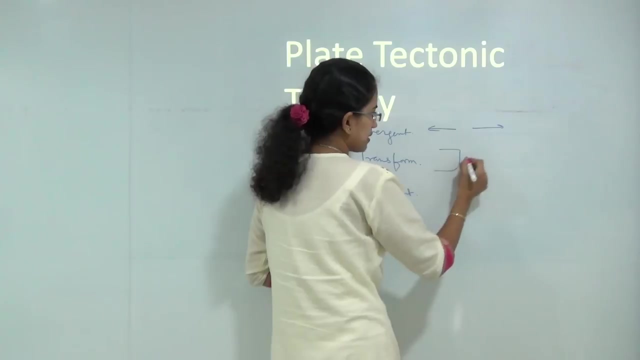 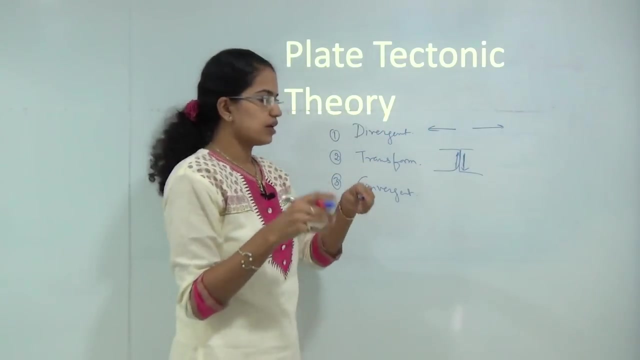 You have the divergent plate boundaries, you have the transform plate boundaries and finally the convergent plate boundaries. Divergent plate boundaries are those plate boundaries which move apart. Transform plate boundaries, I could say, run in a parallel fashion, So it is sliding one over the other. 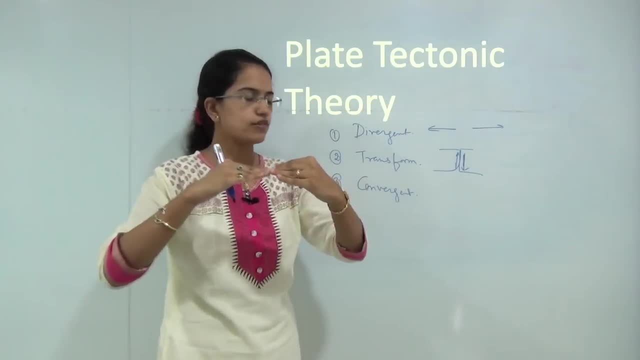 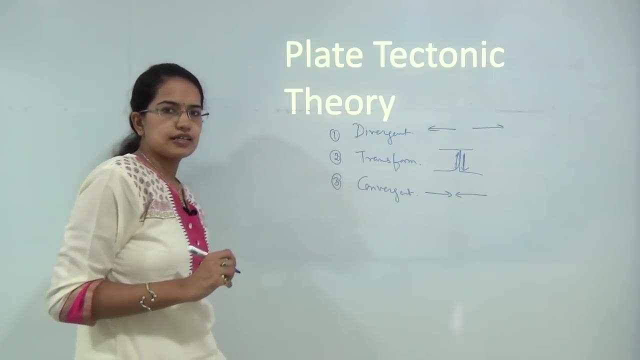 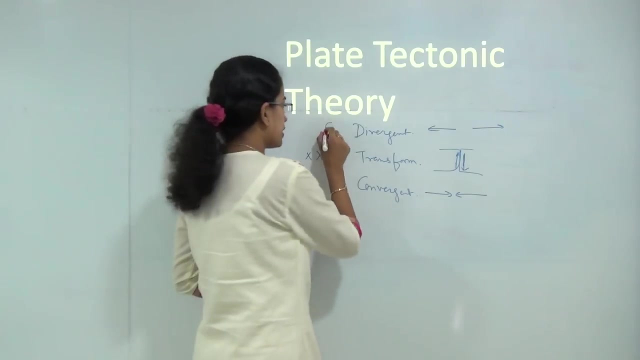 It is diverging, that is moving apart. and finally you have the convergent plate boundaries, which move towards one another. Now, for mountain building purposes, we just ignore out the convergent plate boundaries. Okay, So what we would be including in today's session is the divergent plate boundaries. 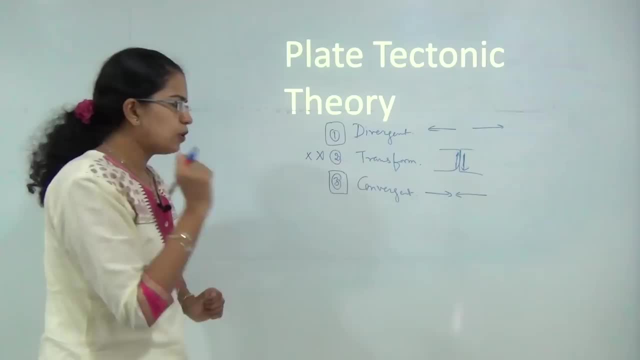 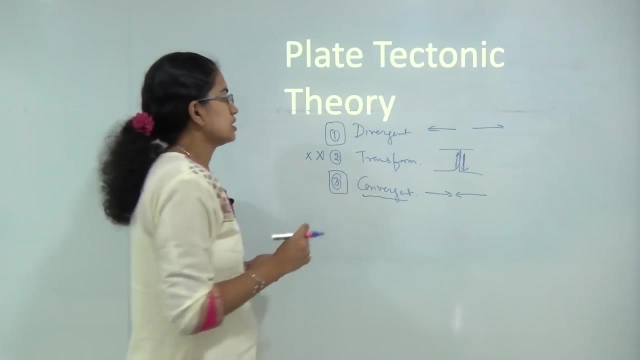 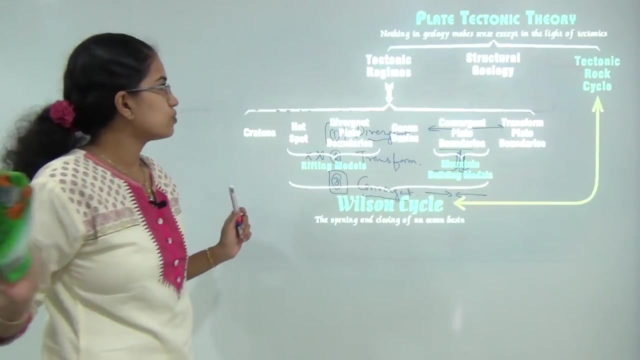 and the convergent plate boundaries. Now, most of the mountains that originated are the result of convergent plate boundaries. We would also understand how divergent plate boundaries lead to origin of mountains. Now let's first start with the basics of plate tectonics. 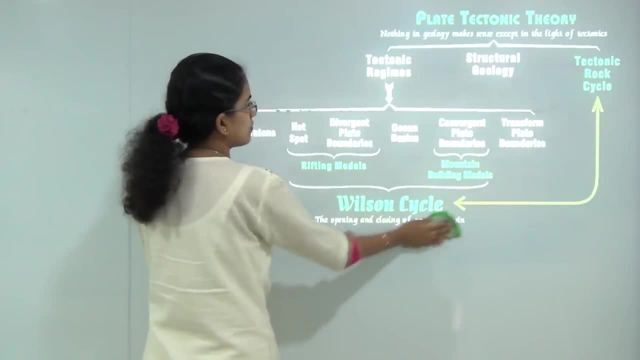 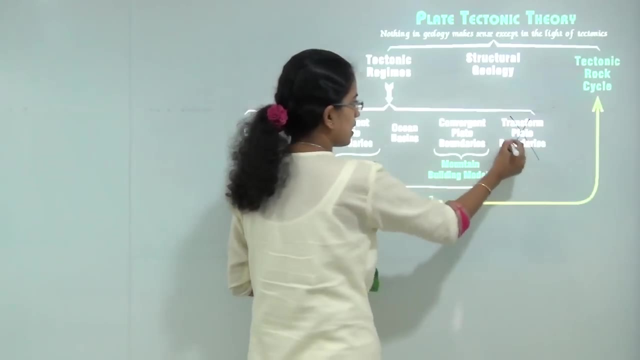 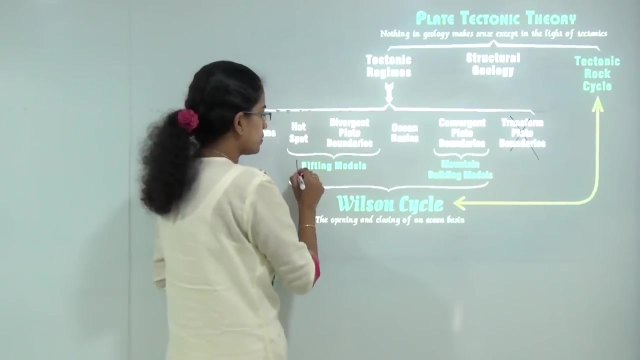 So, as I said, Under plate tectonics you have the divergent, convergent and the transform plate boundaries For mountain building purposes. we are leaving this apart. What we are considering is the hotspots divergent and the convergent zones. The divergent zones are known as the rifting models, while convergent zones are considered. 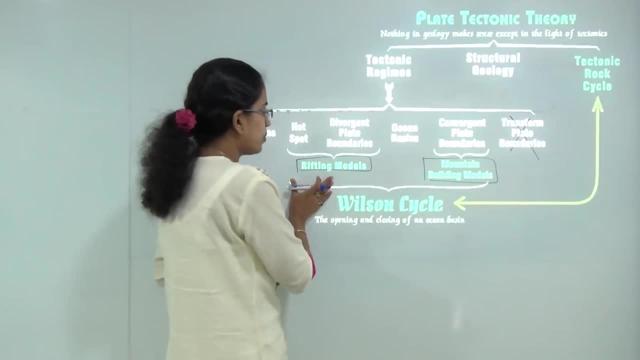 as the real mountain building models, and both these models are covered under Wilson cycle. This we would explain only once, Only when we are done with the real mountain building models. Okay, So let's start with the concept of plate tectonics and mountain building. 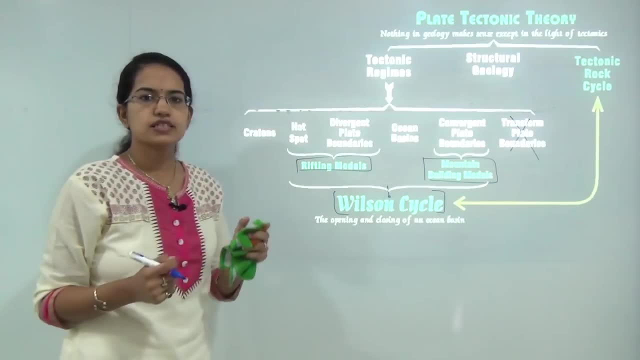 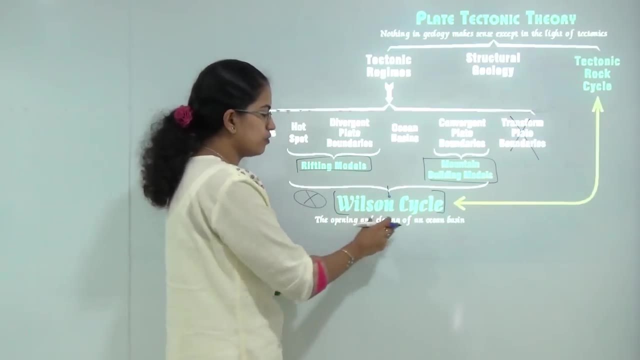 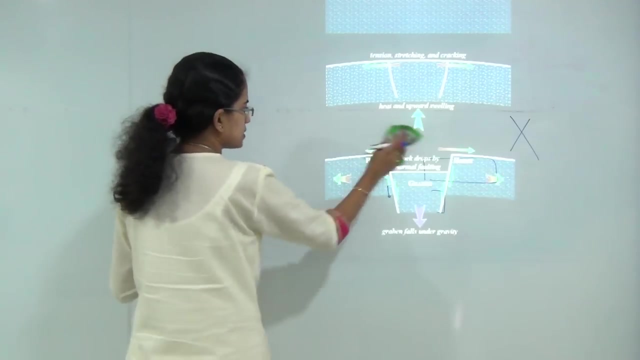 So just for an introduction, Wilson cycle explains the opening and the closing of a ocean basin. So how ocean basin open up and finally close up would be covered under the Wilson cycle. So let's start with the first and the foremost, that is, the divergent plate boundary, or the 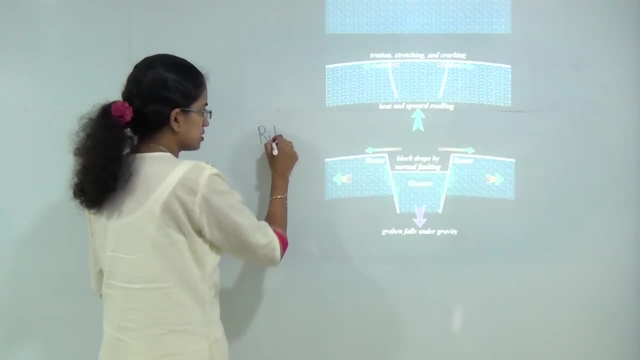 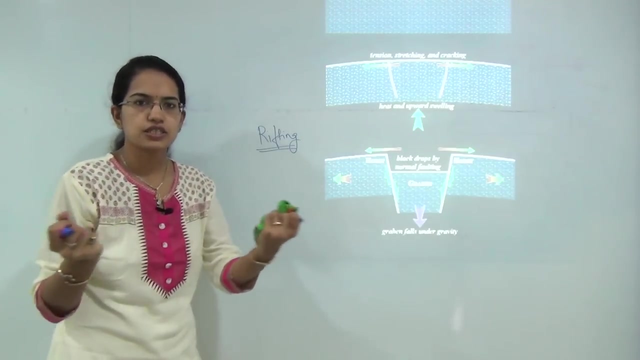 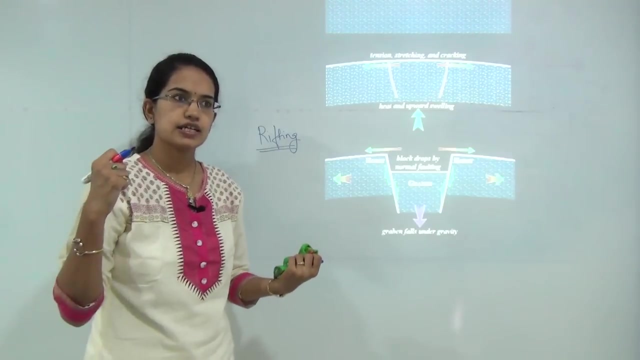 rifting models. So when I say rifting models or divergent plate boundaries, I am trying to explain, Okay, Okay. So I am trying to explain a phenomena that is occurring due to either tension or stretching. So whenever there is tension and stretching, it is a result of either heat or the mechanical 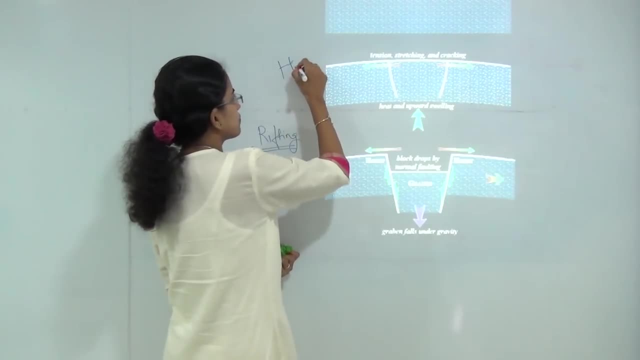 forces that are acting on to it. So for whole of the plate tectonic session, there would be two things that would be important. Either the phenomena would be governed by heat from below, from the core of the plate, Okay- Or the mechanical forces that would be driving it. 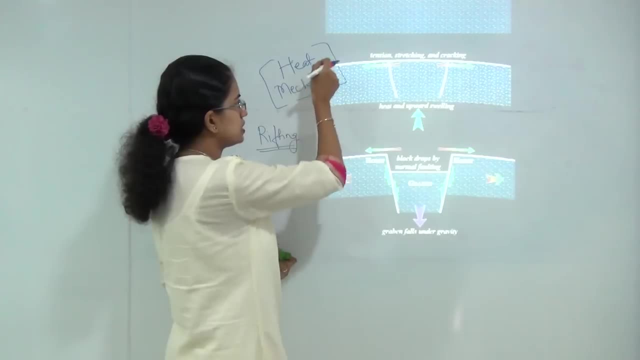 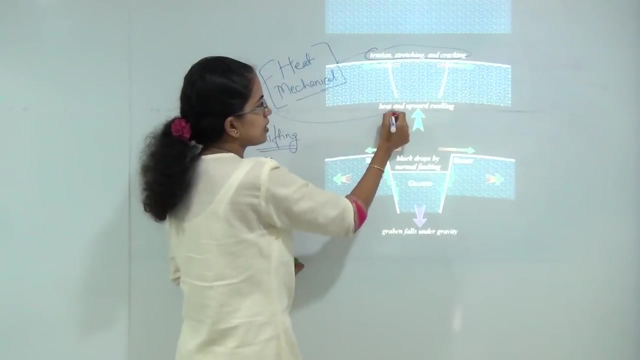 So for now we consider for divergent plate boundaries heat and mechanical action both to act. So tension and stretching and cracking are the result of mechanical action, while heat and upwelling would be the result would be heat driven from the interior of the earth. 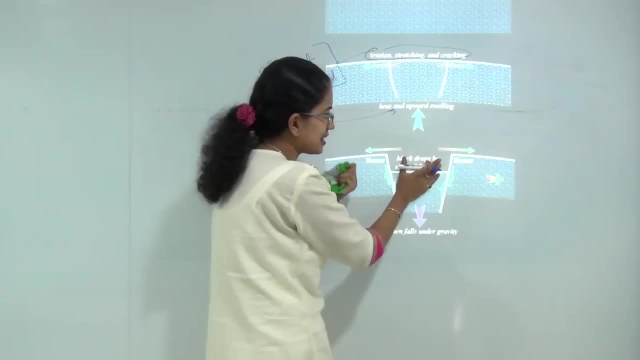 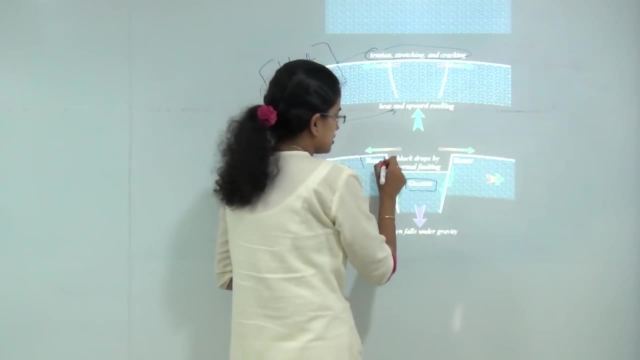 These lead to stretching and, finally, what happens is the center block drops down, and this region is the center block, Okay, Okay, So this region is known as garban. The surrounding region which remain up at a higher level are known as hollest and the. 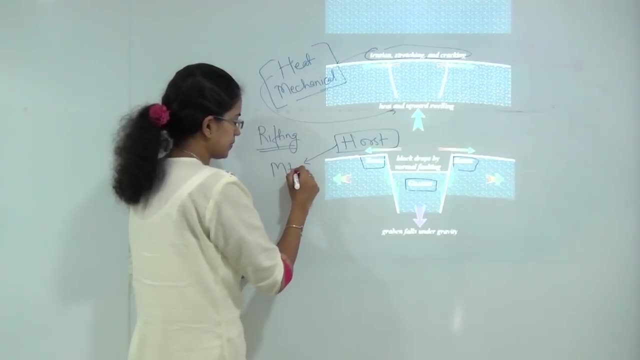 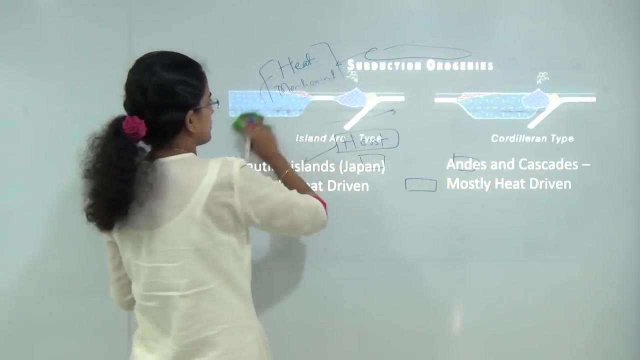 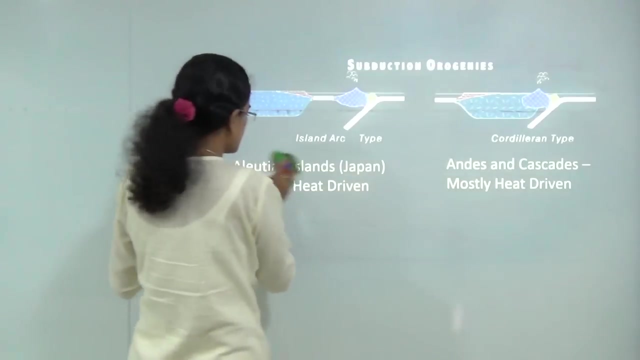 divergent plate boundaries result in the formation of hollest mountain. So that is one thing. Now we will move on to convergent plate boundaries. When I talk about convergent plate boundaries, when anything is converging, there can be two thing that is happening. 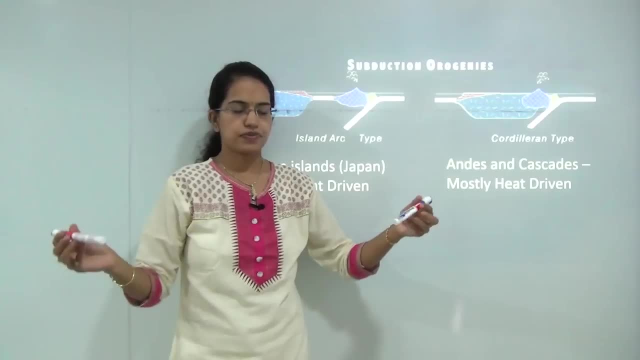 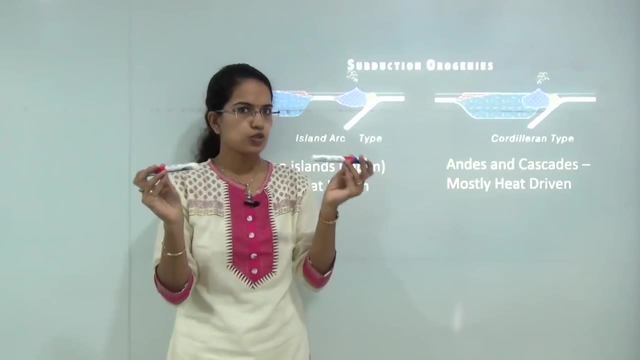 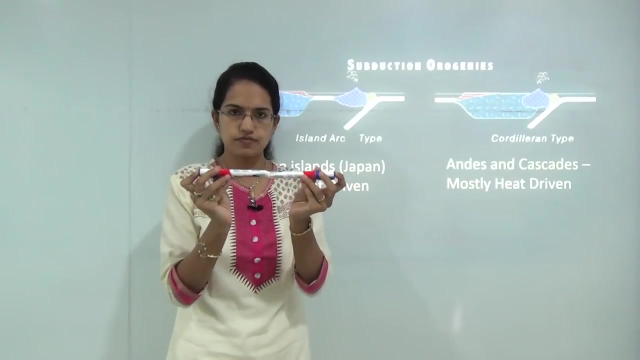 So you have two pens here and what is happening is they are converging or coming close to one another. So there can be two phenomena that can occur. one is a head on collision, So what we would explain is a collision phenomena, and next is this: which is weaker might get. 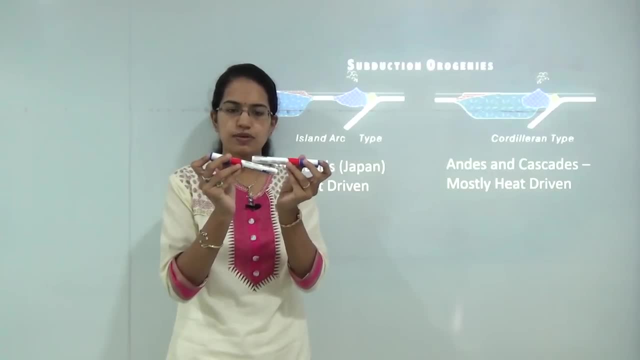 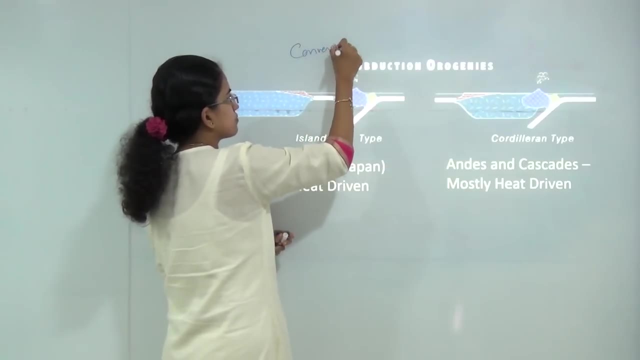 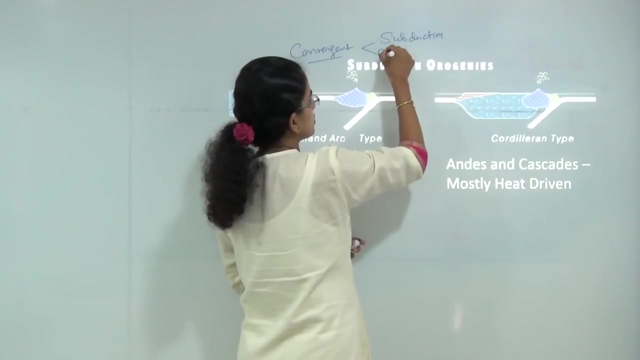 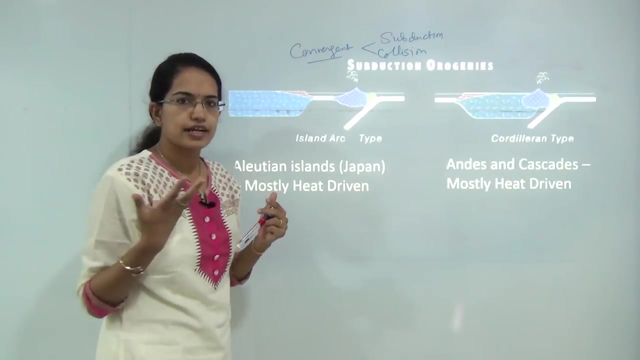 subdued under this, or there can be a force of subduction that acts okay. So there would be two things under convergent plate boundaries that we would try to understand. one is subduction and other is collision. Now our earth is made up of both continent and water. 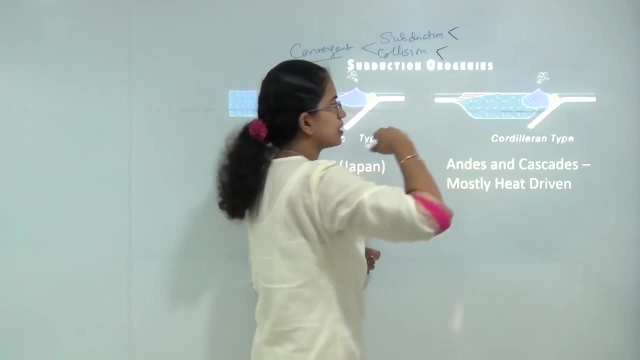 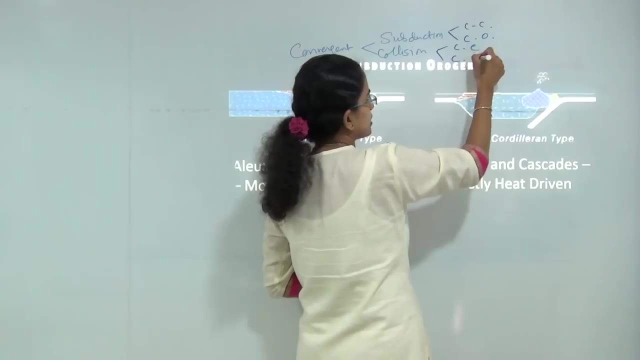 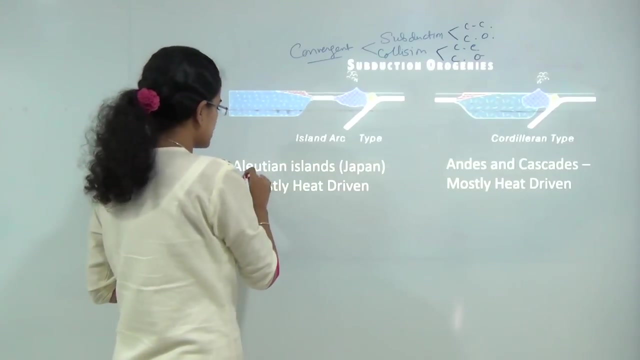 So you have for both of these cases. we would further take two cases, So you would have continent-continent, continent-ocean, continent-ocean, continent-ocean, continent-ocean, continent-ocean. Now, when we talk about subduction, you have an island arc here. a classic example would: 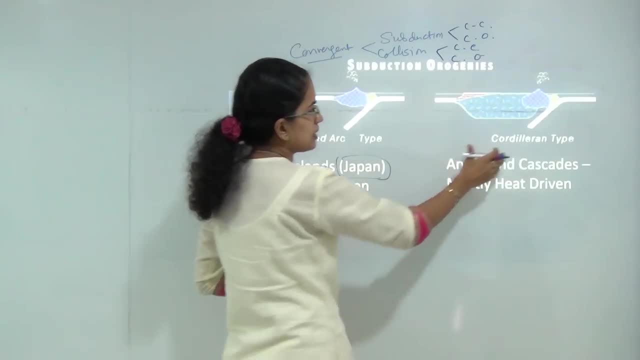 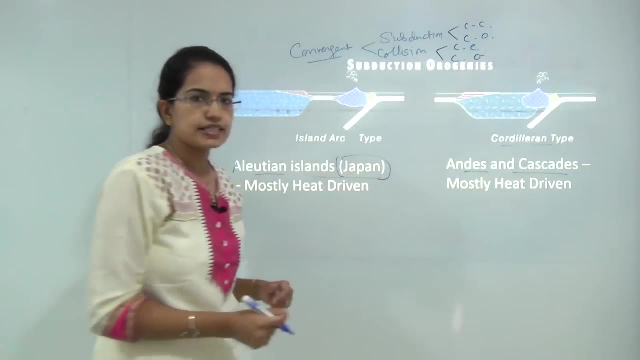 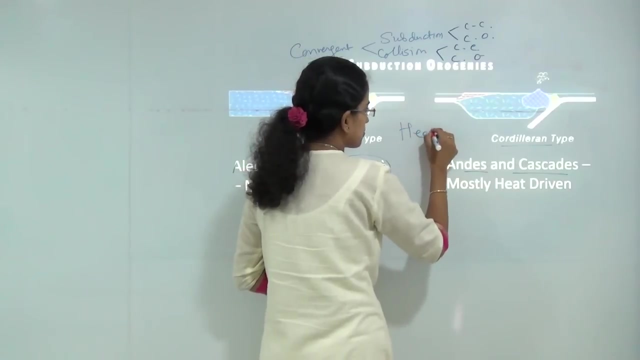 be Eltusian island group in Japan and you have a cordylerian type where you have parallel series of mountains. here the classic example would be Andes and Cascade ranges. under both these phenomena, where there is subduction acting, the primary force here would be heat. 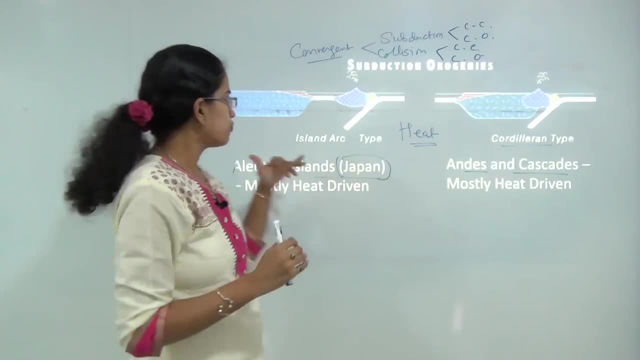 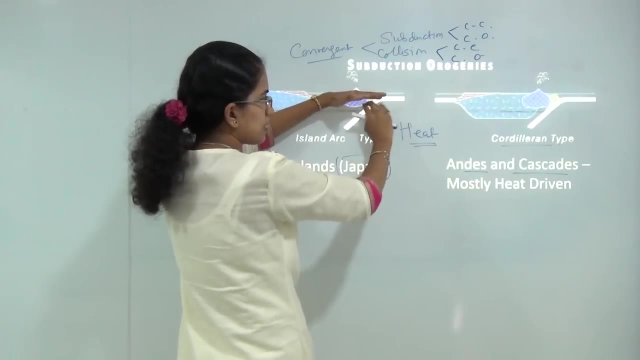 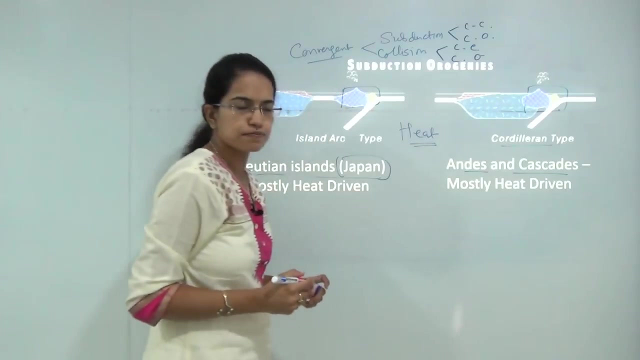 So subduction forces are usually heat. So you have one block and the other block get subsided below this block and there is where there is the region of subsidence or subduction. you would have the process of mountain building that originates here. So that is what is the subduction originate. 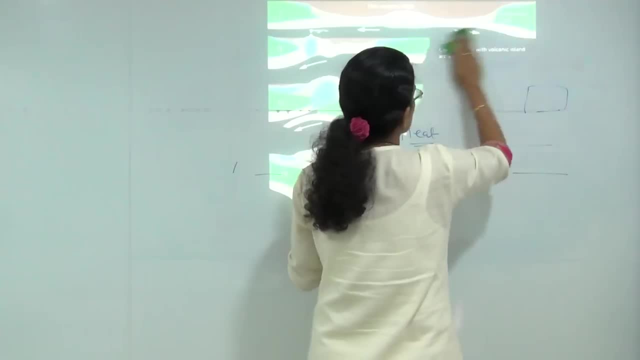 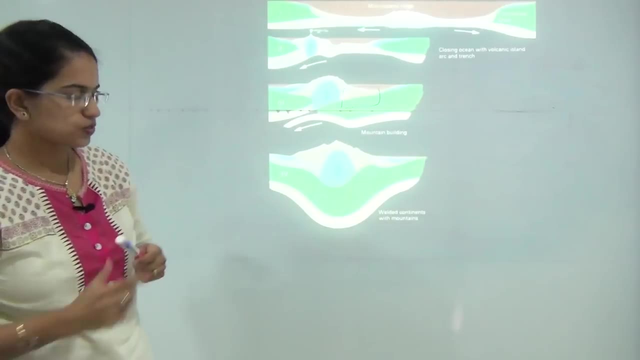 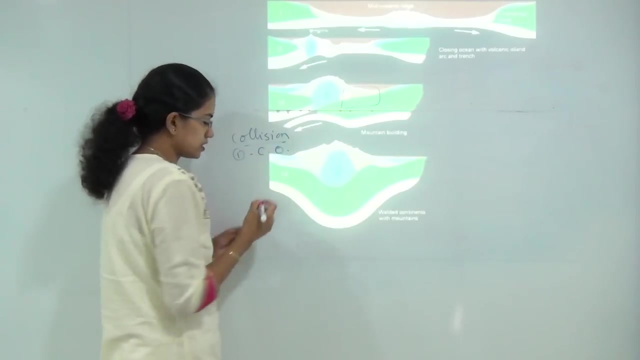 The next we would try to understand is the continent-ocean for collision. So we talked about subduction. The next was collision. So under collision we would be taking the first case of continent-ocean convergence. So when there is a convergence of continent and ocean, what happens? 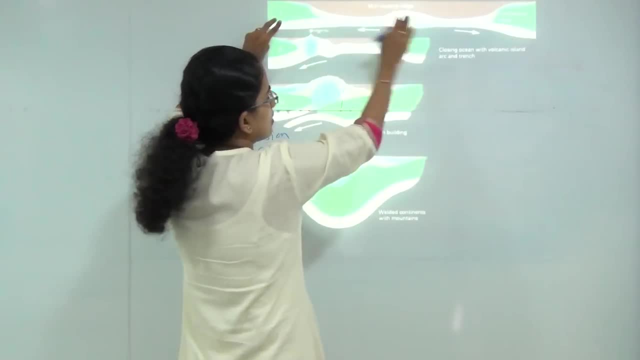 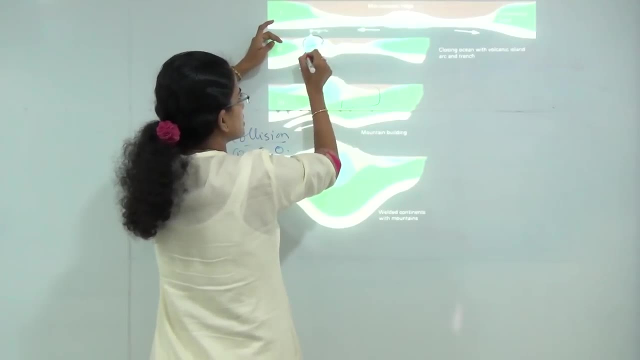 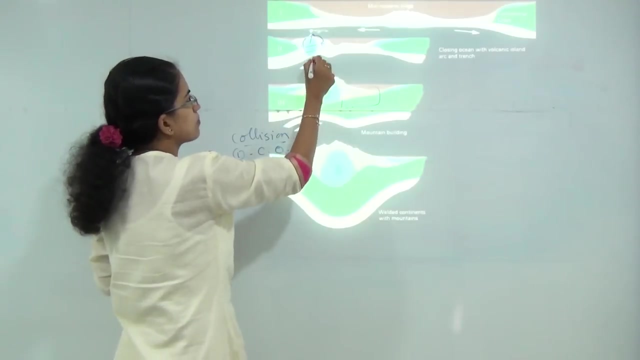 You have a ocean region, you have the mid-Atlantic region and you have the coast here. So there is kind of collision that ends. The point where the collision occurs is the region for the initiation of mountain building process. So you have the mountains that are coming up, the heat that is coming up along with. 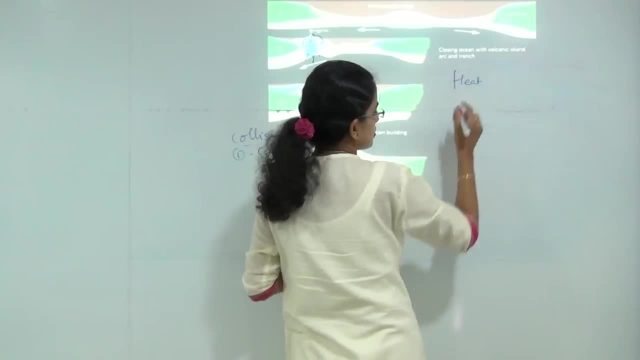 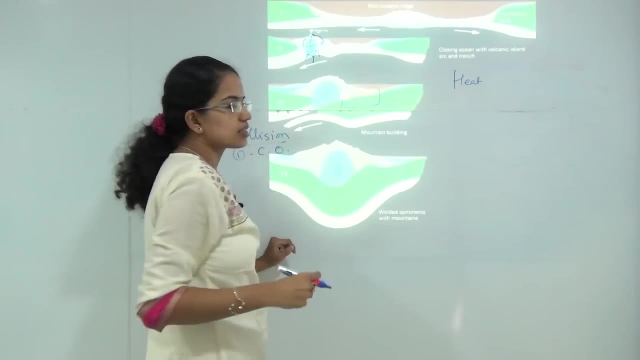 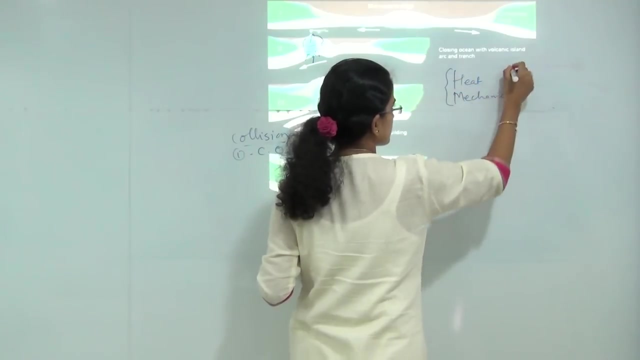 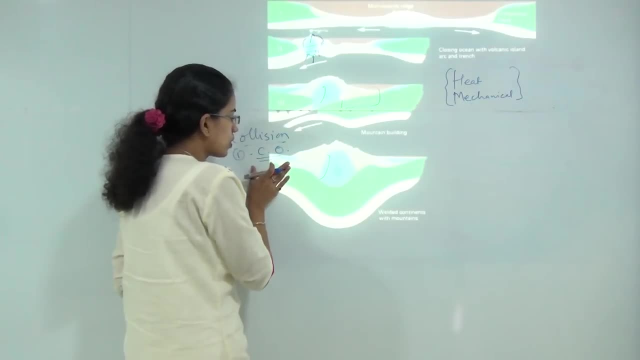 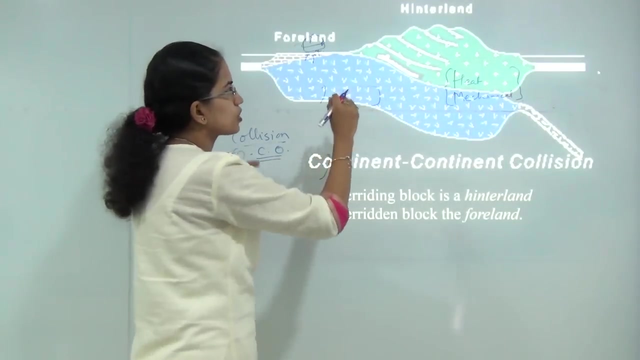 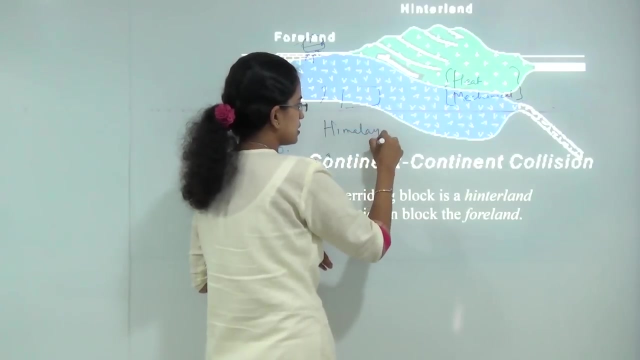 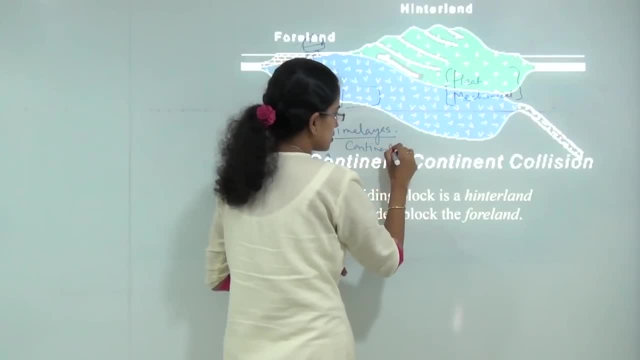 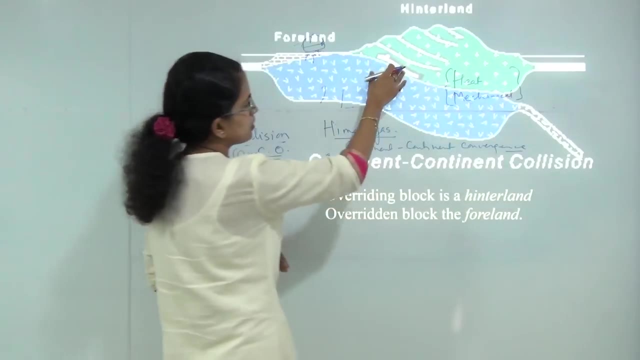 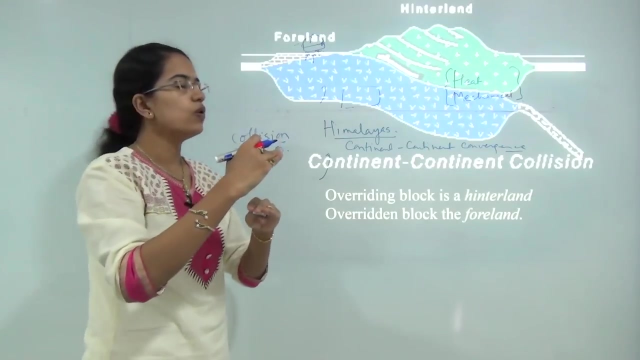 convergence. So you have continental land mass on both the sides And due to the process of convergence here you have the formation of Himalayan mountain. Now here there are two blocks: one is the foreland and another is the hinterland. So hinterland is the overriding block, that means which is riding above the existing mass. 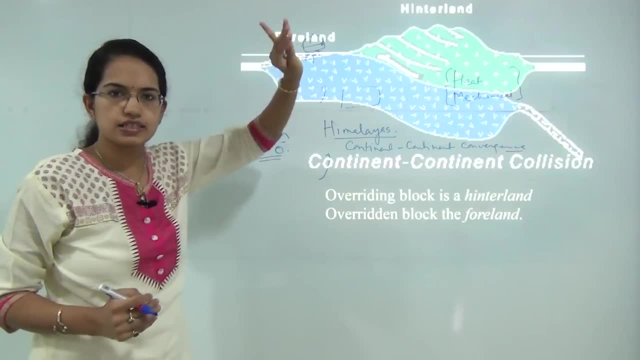 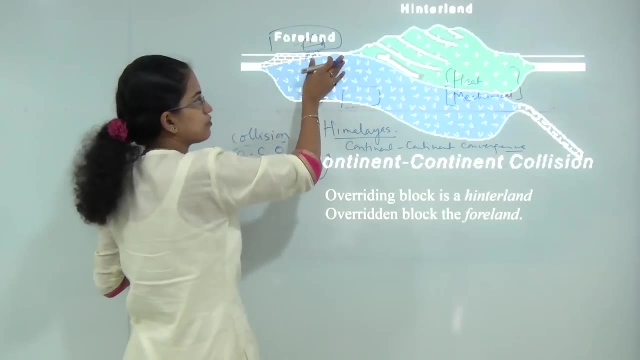 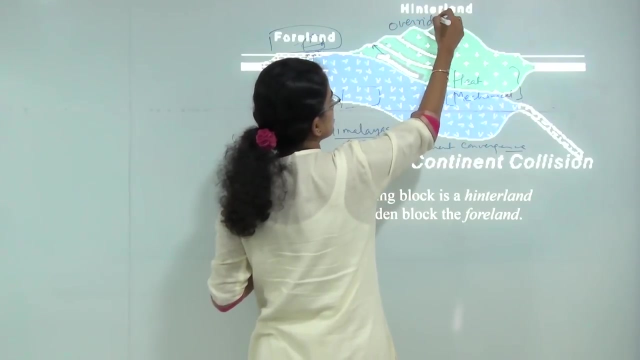 while as foreland, which was considered as a rigid mass under cobers theory, is again a overridden block here, because this remains kind of rigid and this is the mobile or the moving mass. So this is, I could say, the overriding mass and this is the mass which is overridden. 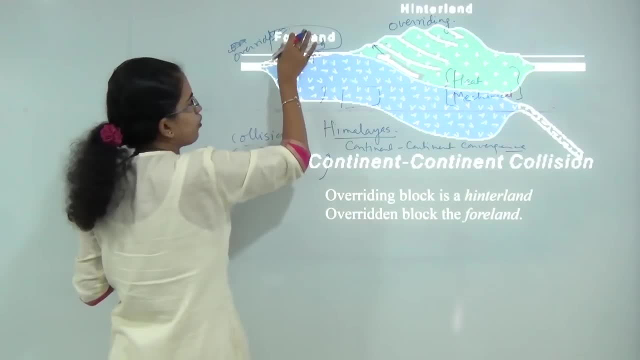 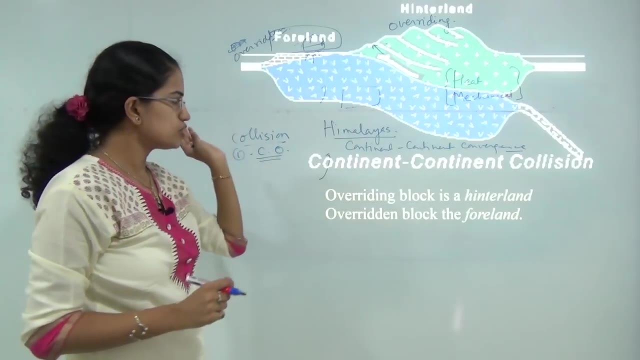 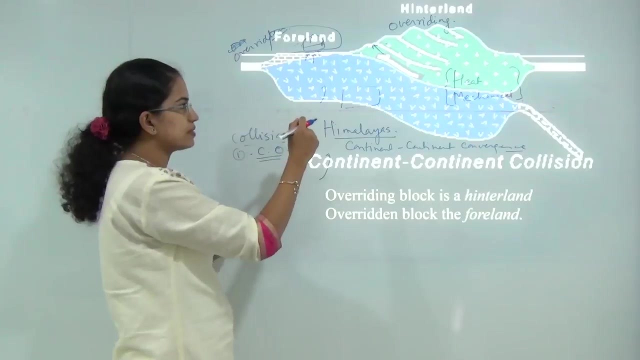 So it is a overridden mass. So foreland would be a overridden mass. in contrast to that, hinterland would be an overriding mass. So these are the various concepts that we try to understand under the plate tectonics theory and how mountain building process takes place under plate tectonics. 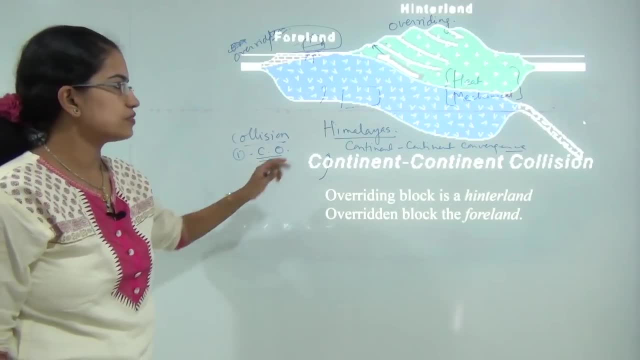 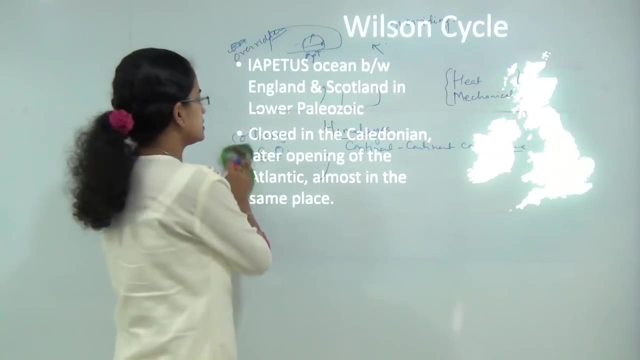 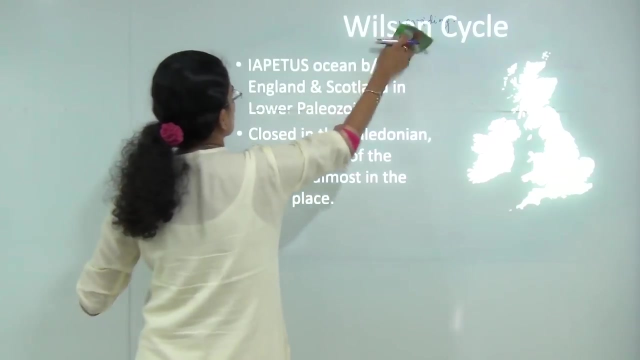 Now let us move on To another interesting concept. once we have completed the plate tectonics theory for mountain building, we can very well appreciate the concept of Wilson cycle. Now, to start with, why Wilson cycle originated. It was given by Tuzo Wilson, who lived from around 1908 to 1993, and it is a kind of a 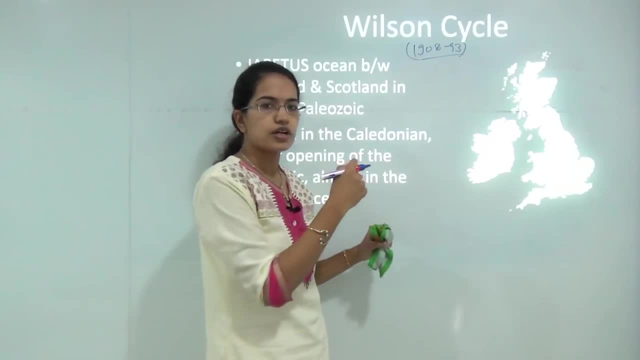 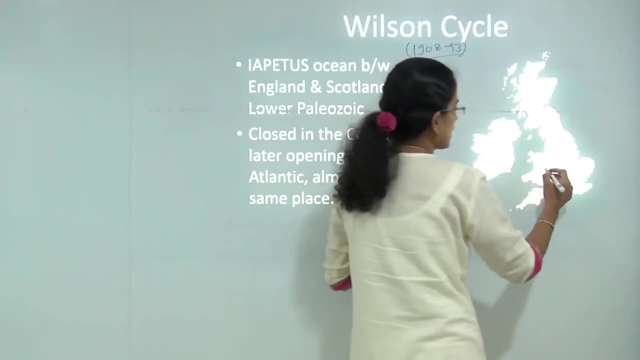 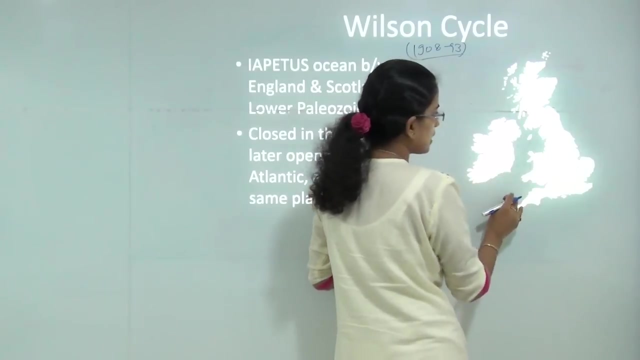 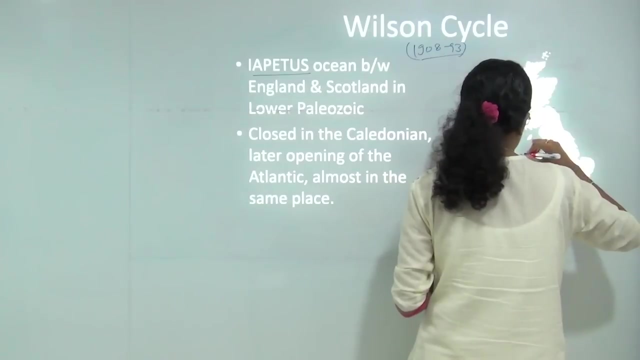 very recent concept in the field of geomorphology, in contrast to the other theories that have started. So where he started was the region of England and Scotland. In the region of England and Scotland he tried to explain. the intermediate ocean between the two regions was known as Apeteus. 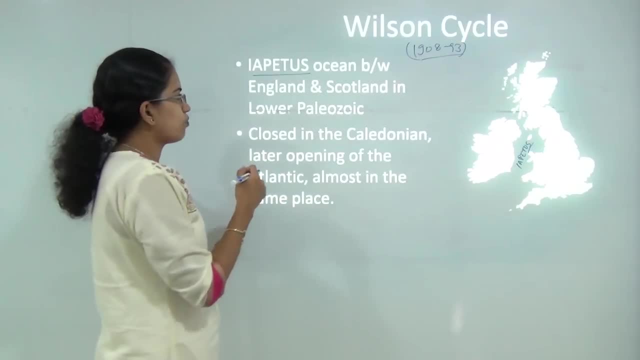 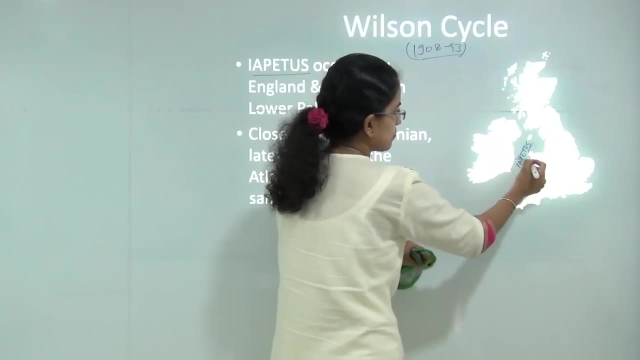 What happened during the Cladonian phase was: this ocean got closed up. Finally this ocean got closed up. Finally this ocean got closed up. Finally this ocean got closed up. So that was a kind of common landmass that establish here. this ocean got closed up and 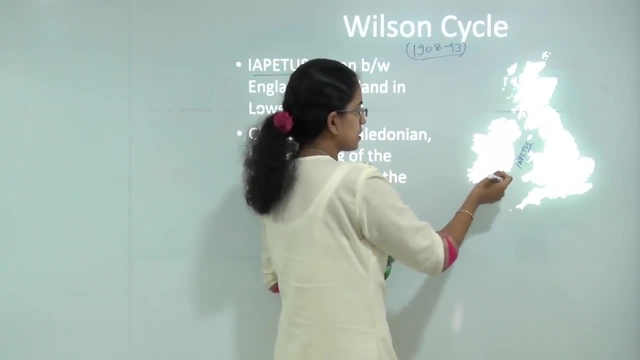 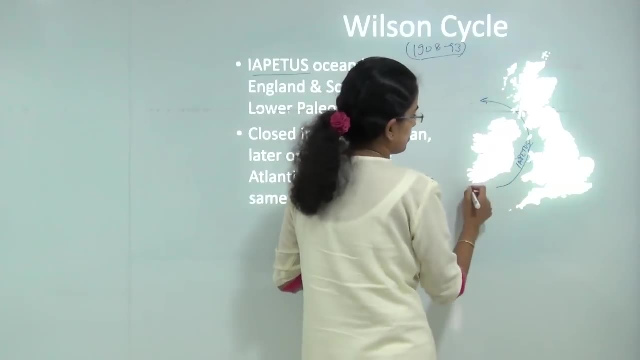 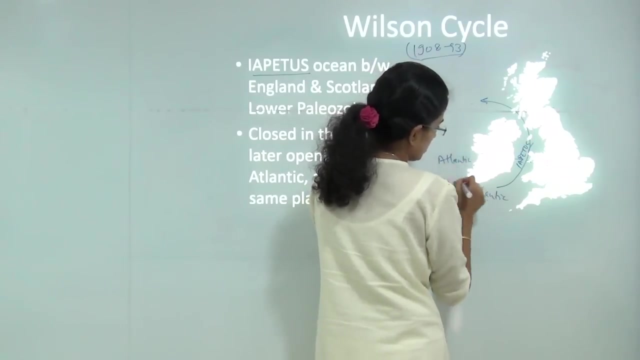 finally, what happened was during the period of later Paleozoic, this region again opened up to Atlantic Ocean. So you had atlantic ocean here and again there was a region that opened up here, which was the extension of the Atlantic ocean. Now let us do another deep Lessons. 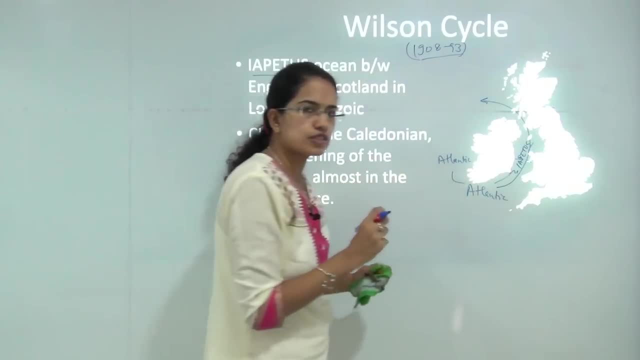 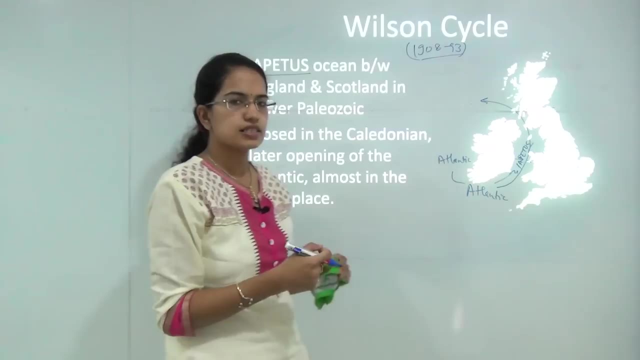 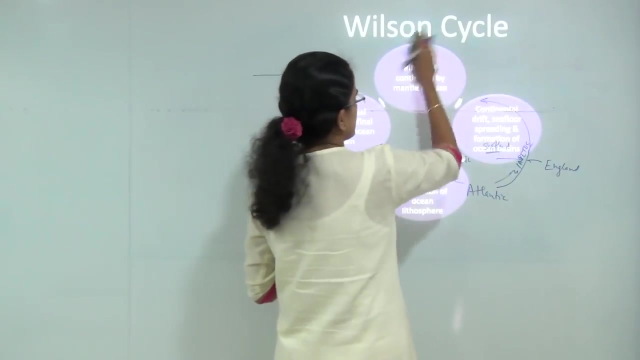 After learning about Pleozoic related questions and get」 Atlantic Ocean. Now, why this happened was the main idea that led Tuzo Wilson to research more, and when he researched, he gave this concept as Wilson cycle and what he propounded was an interesting phenomena. He said we will move on to this diagram later. let us try to. 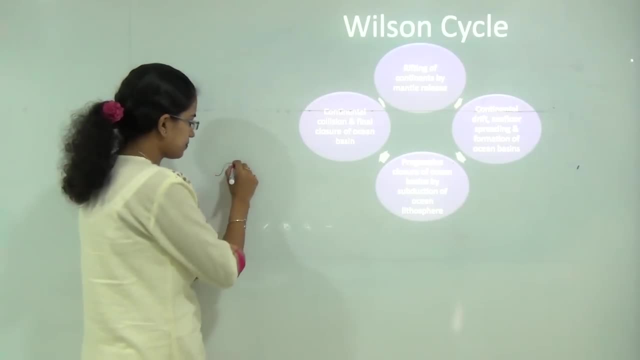 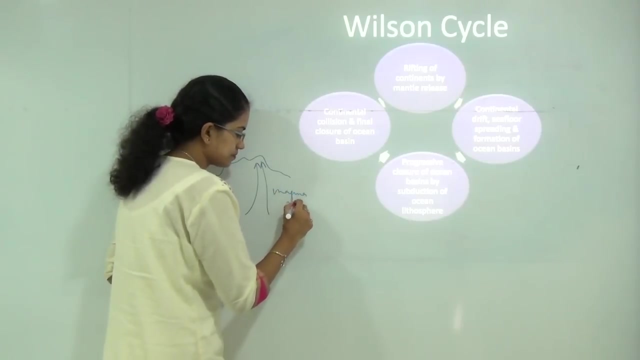 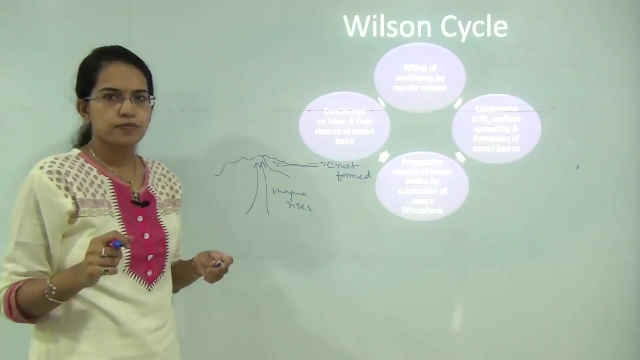 understand it by ourselves first. so you have the volcanoes. what happens is there is magma that rises. Once the magma rises here, what happens is this magma flows on the surface and you have the formation of crust. this crust is formed, so hot magma comes from inside, spreads. 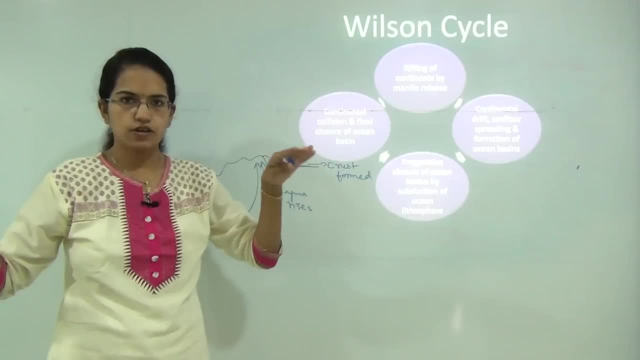 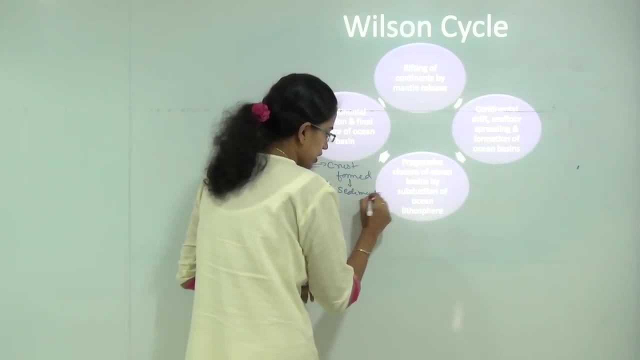 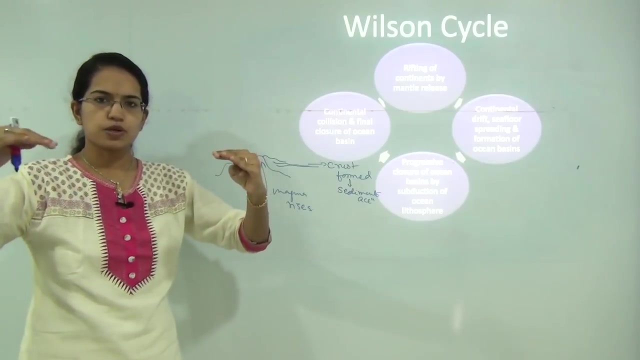 on to the top of the volcano. this is called magma top of the earth, which leads to formation of crust. this formation of crust is accompanied by accumulation of lot of sediments, so I could say sediments get accumulated here. once the sediments are accumulated, there is process of subduction that occurs at one end and on. 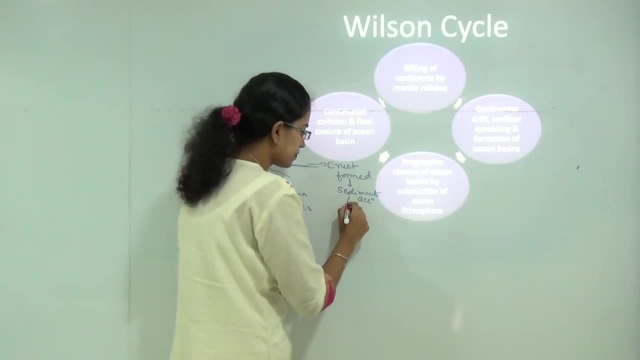 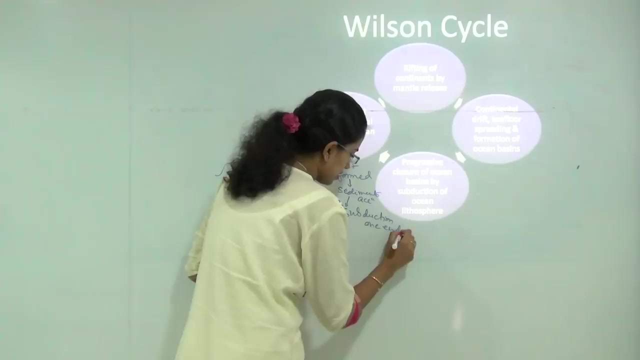 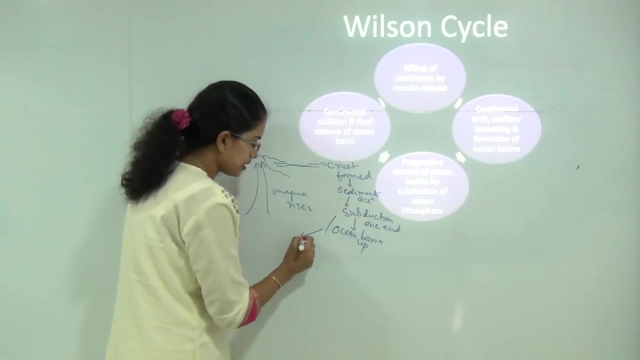 the other end you have the ocean basin that closes up, so you have subduction that occurs at one end and you have the ocean basin that opens up at the other end. so what results in this would be again crustal thinning, and this crustal thinning would again go back. 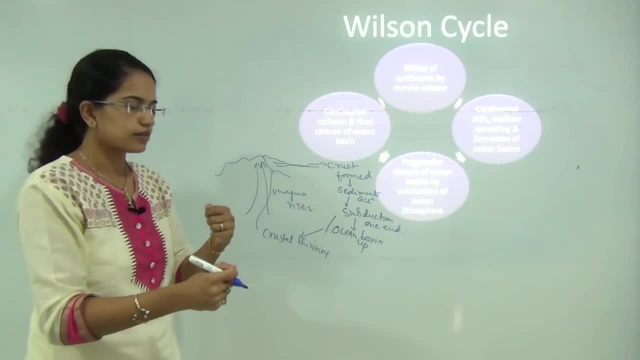 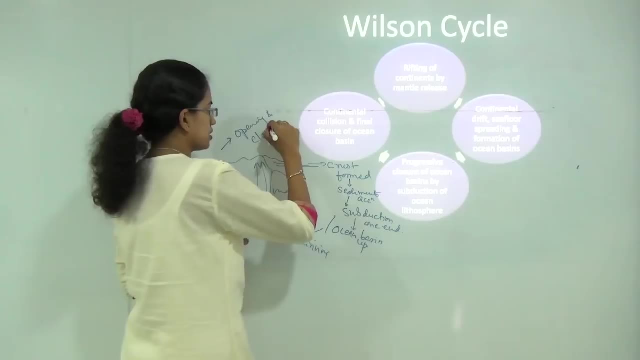 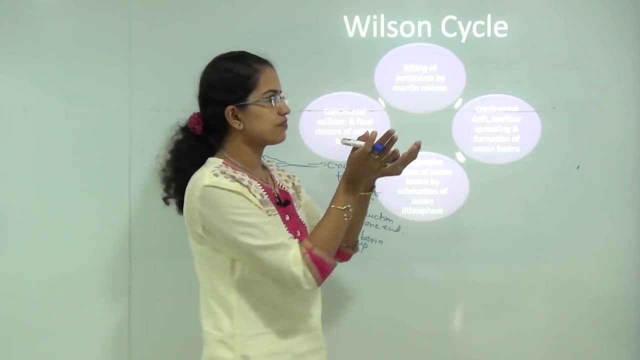 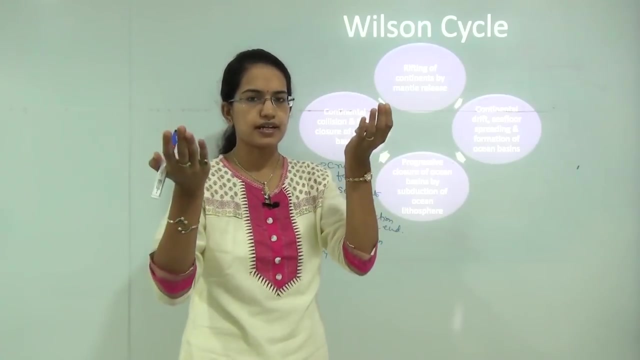 so it's a kind of cycle that continuously goes on And we have compounded this cycle as the opening and closing of the ocean surfaces. so what we try to understand here is: let's try to see here: so you have rifting of the continents by mantle, so the hot magma and mantle comes. hot magma comes from inside the mantle and 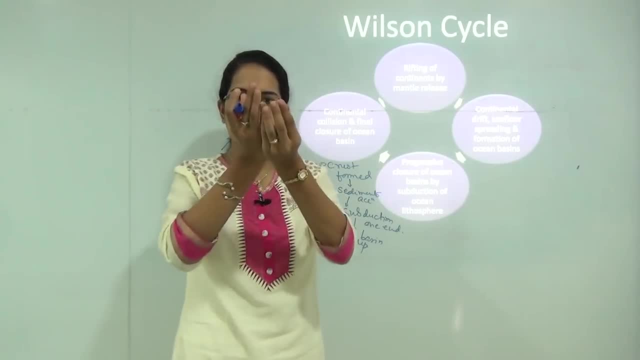 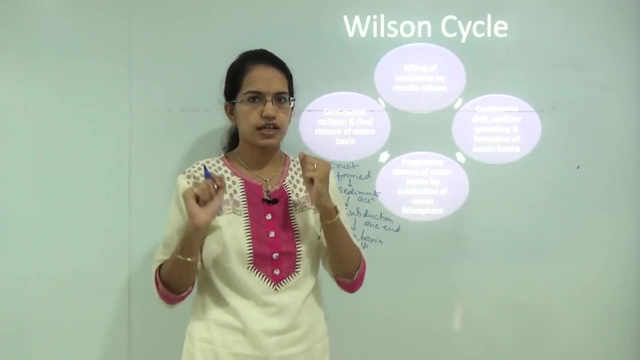 you have the rifting of the continents, so the point where the magma comes in the continent moves apart. what would happen is this would result in the rifting of the continents and theőlison for description. Now, this is rifting, so what would happen is the the abondance of the continents goes.